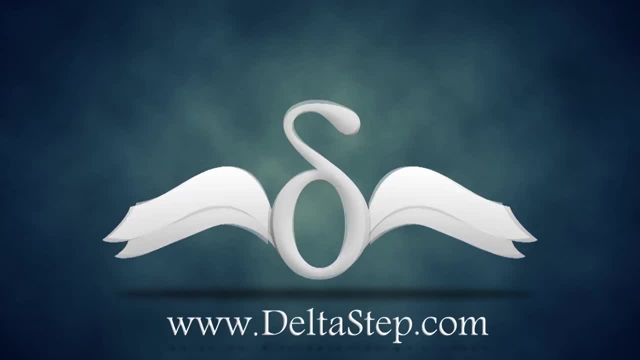 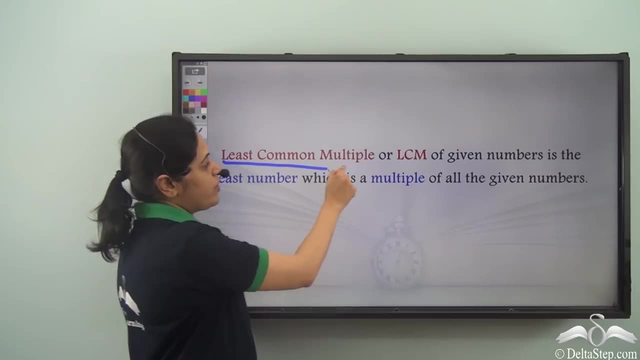 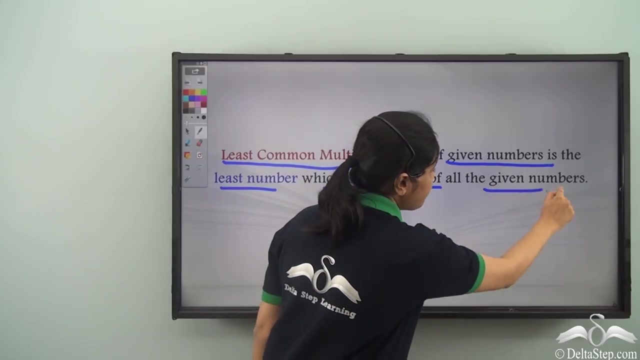 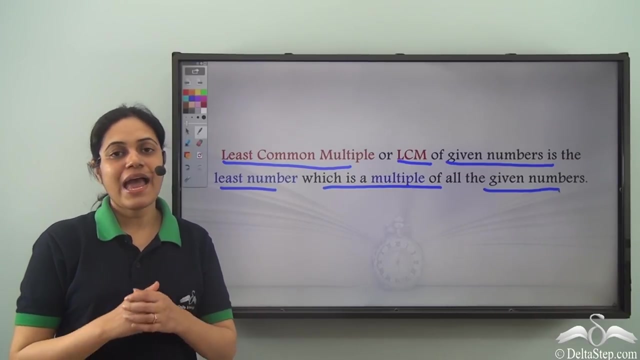 You have already learnt what is LCM: Least common multiple or LCM of given numbers is the least number which is a multiple of all the given numbers. So a number which is a multiple of all the given numbers and the smallest such number. We have also learnt. 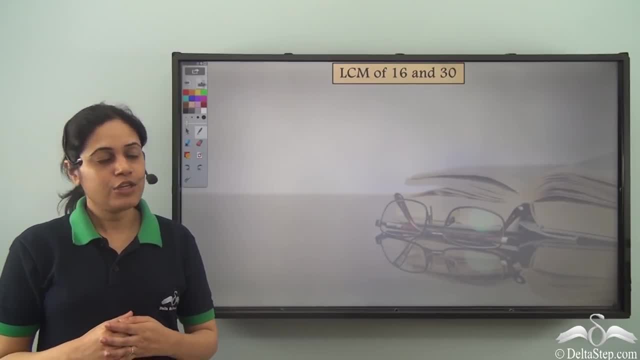 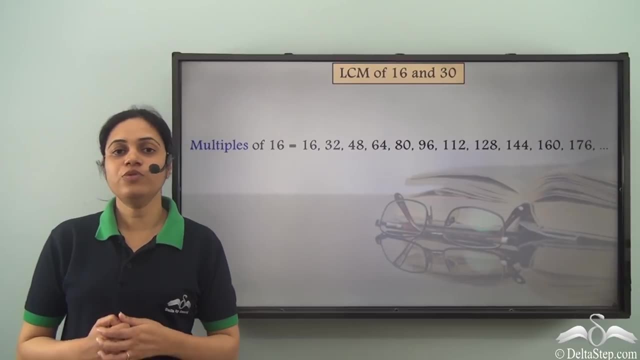 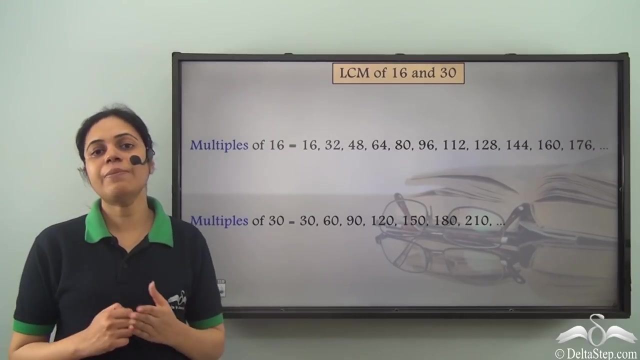 how to find the LCM using the listing method. So suppose I want to find the LCM of 16 and 30. So first I need to list down the multiples of 16. So these are the multiples of 16, and then I need to list the multiples of 30, and now I need to find the LCM of 16 and 30. So 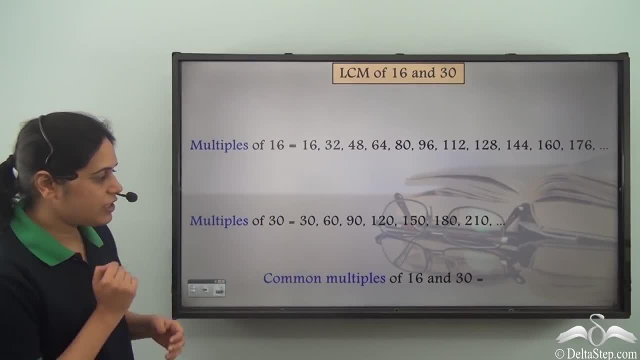 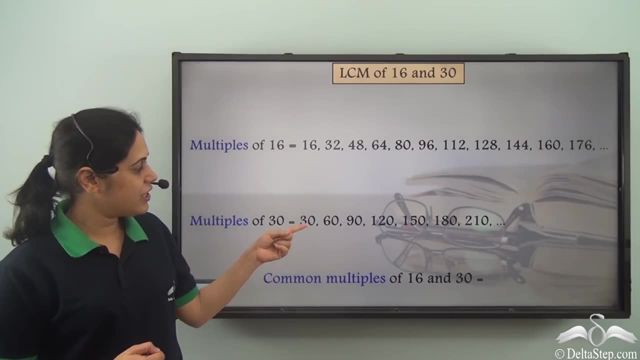 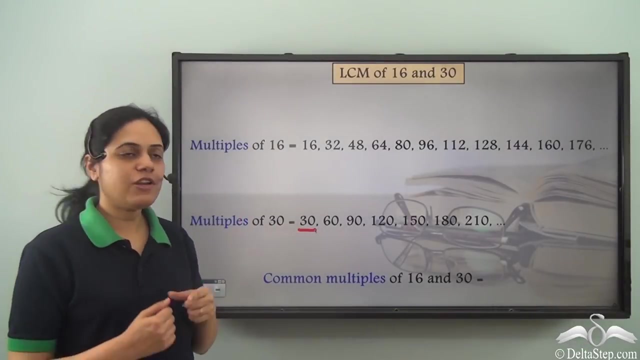 now I need to find the common multiples. So let's find the common multiples. How do I find the common multiples? I take different numbers and see whether the number is present in the other list as well. So I start with 30. Is 30 a multiple of 16? No, What about? 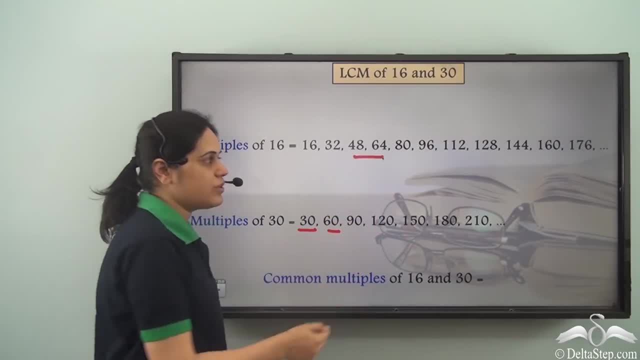 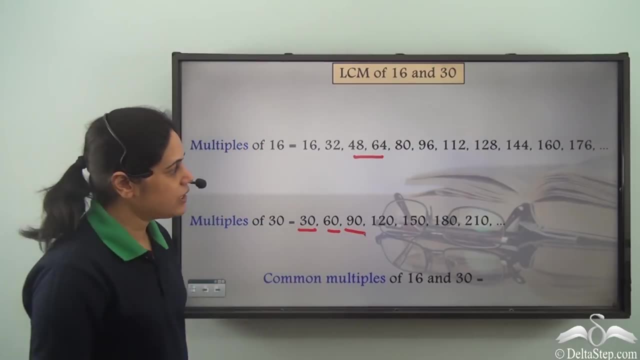 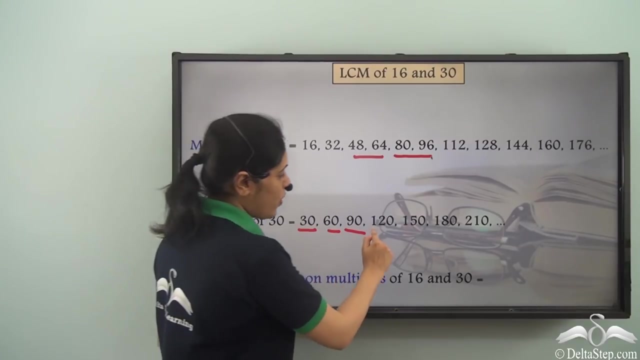 60?? Is 60 there in this list? No, So 60 is not a multiple of 16.. 90 is a multiple of 30, but 90 is not there in this list, So 90 is not a common multiple. 120 is there in. 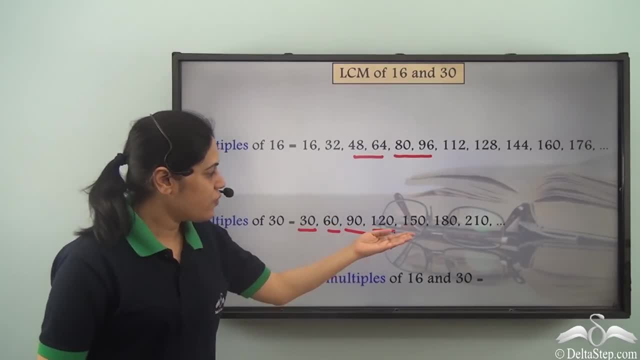 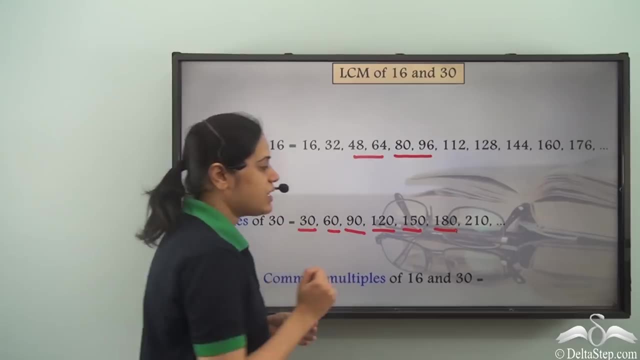 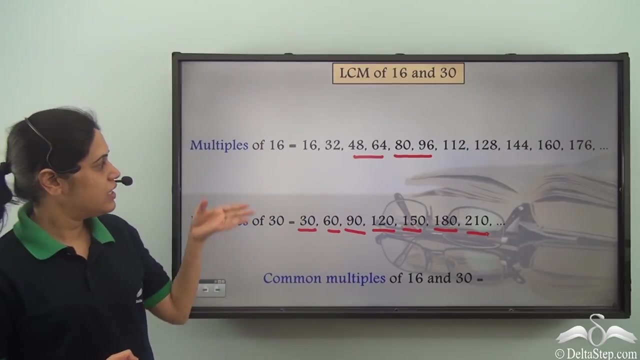 this list, but it's not there in this list. 150 is there in this list, but it is not a multiple of 16.. 180 is a multiple of 30, but it is not a multiple of 16.. 210 is a multiple of 30. 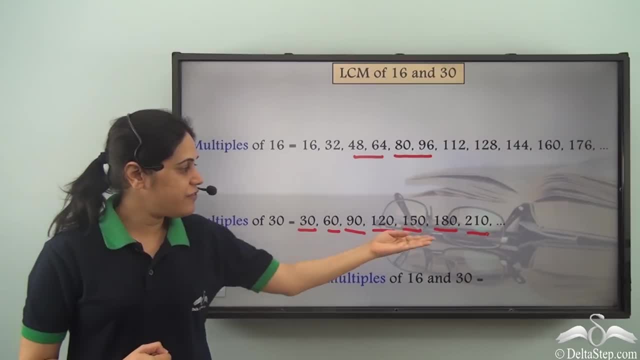 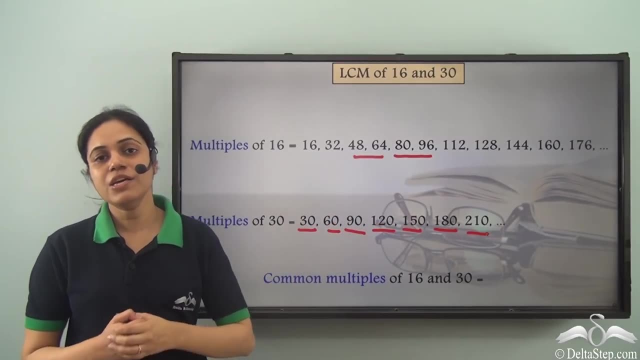 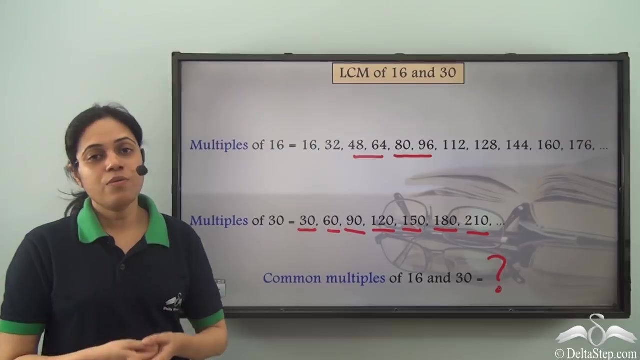 but it is not a multiple of 16.. So see, I have reached till 210, which is a big number, but still I am unable to find a common multiple. So I am unable to find a common multiple. Now, the disadvantage of the listing method is this itself: 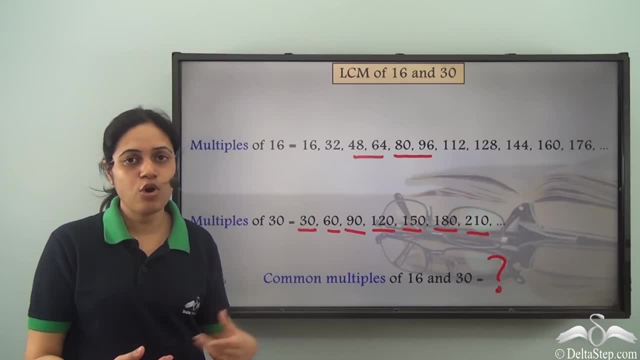 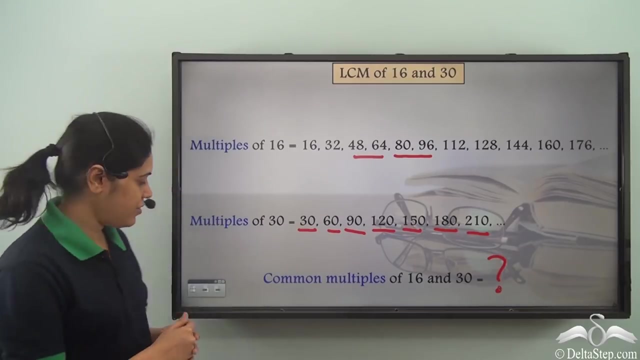 I don't know till what number do I have to go to find the least common multiple or the LCM? So it is very time consuming. Do we have a simpler method to find the LCM? Yes, fortunately we do have This. method is known as the prime factorization method. 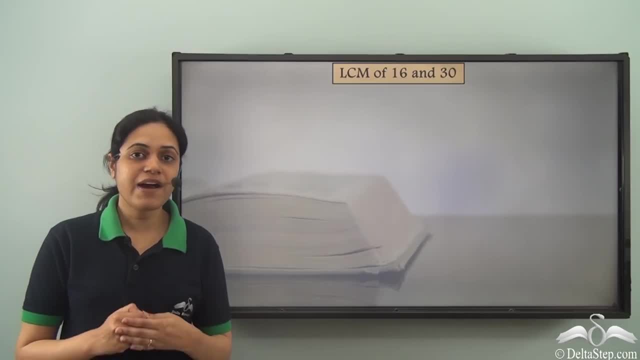 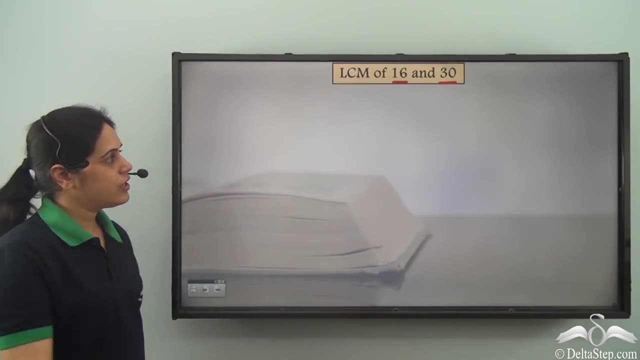 So, as the name itself suggests, in the prime factorization method I need to prime factorize 16 and 30. Now how do I prime factorize 16?? So I start dividing by the lowest prime number possible, so which is 2.. 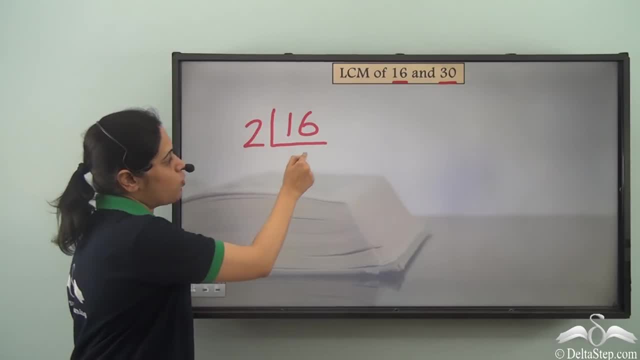 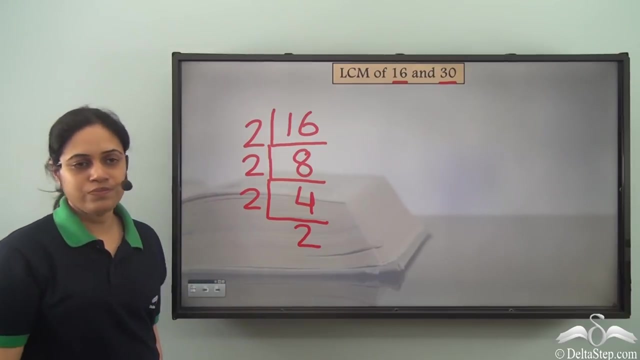 So 16 is divisible by 2. The quotient is 8. So I write the quotient here Once again. I divide 8 by 2 to get 4.. I divide 4 by 2 to get 2.. And again I divide 2 by 2.. 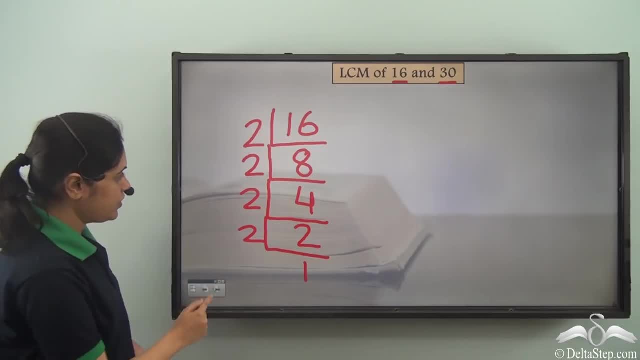 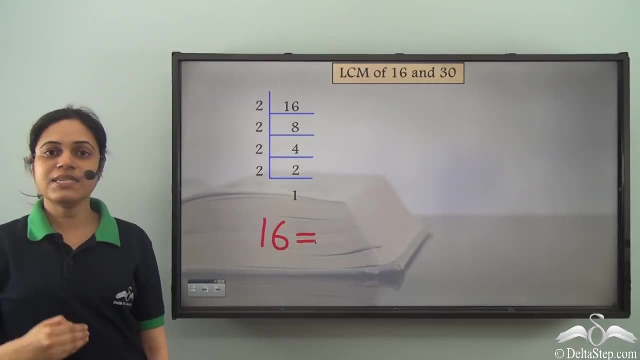 2 to get 1.. So I stop when I get 1.. So this is what I have. So I can write 16 in terms of its prime factors. How 2 into 2, into 2 into 2.. 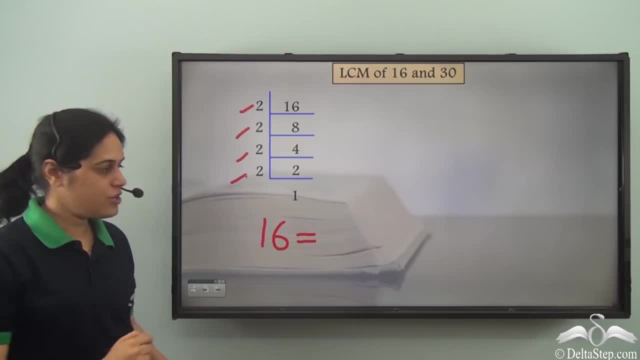 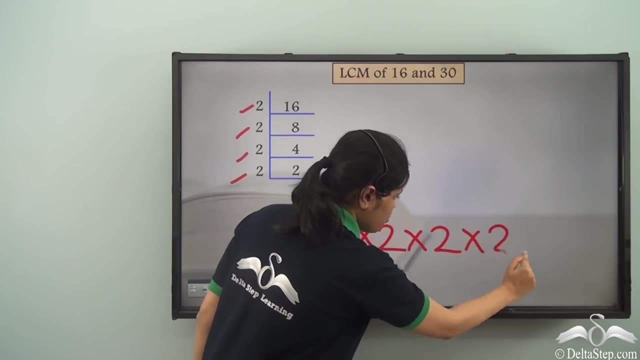 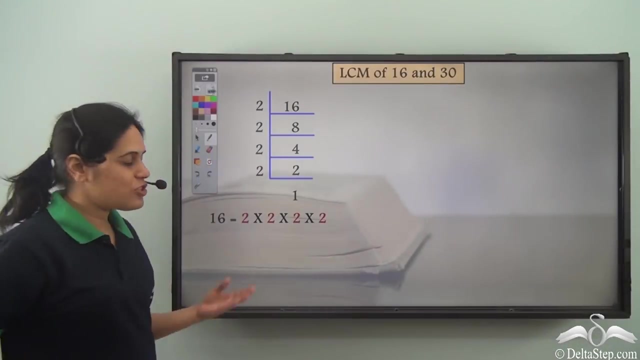 These are the divisors. So I have 2 four times. So I can write 16 as 2 into 2, into 2, into 2.. So 2 multiplied by 2.. 2 multiplied 4 times because I have 2 four times here. 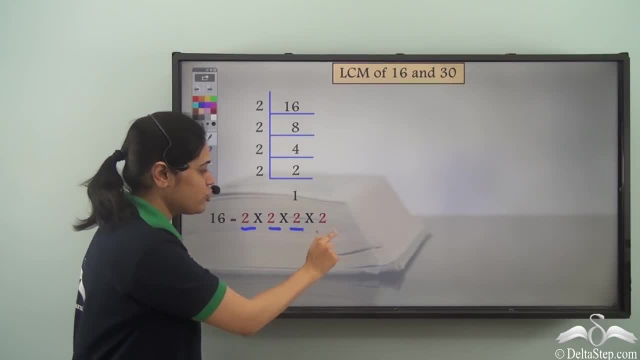 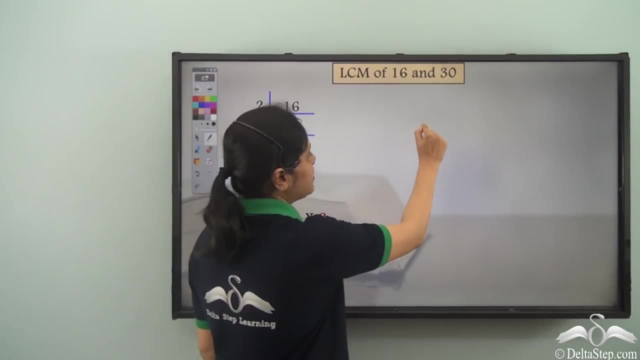 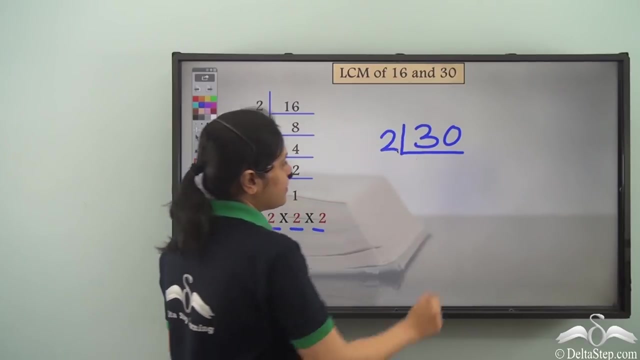 So 16 can be written as 2 into 2, into 2 into 2.. That is 2 multiplied 4 times. Now, similarly, we need to prime factorize 30 as well. So I will divide 30 by 2, because that is the lowest prime number and 30 is divisible by. 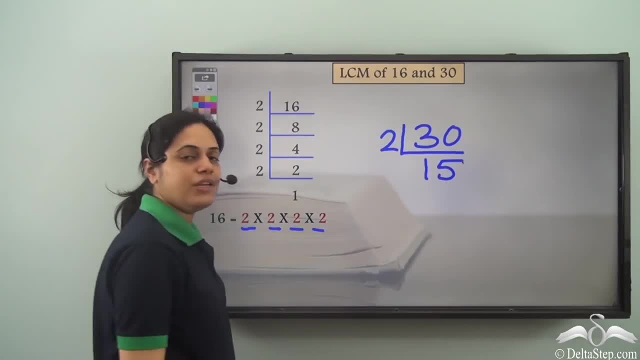 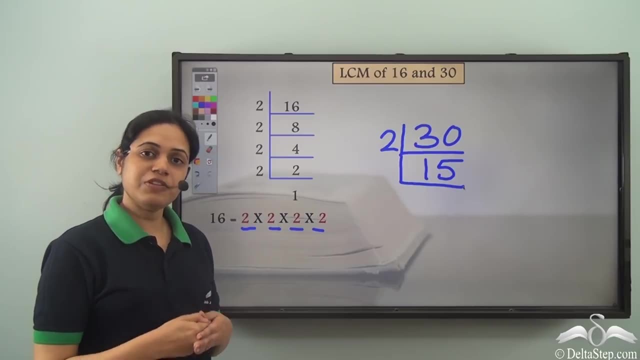 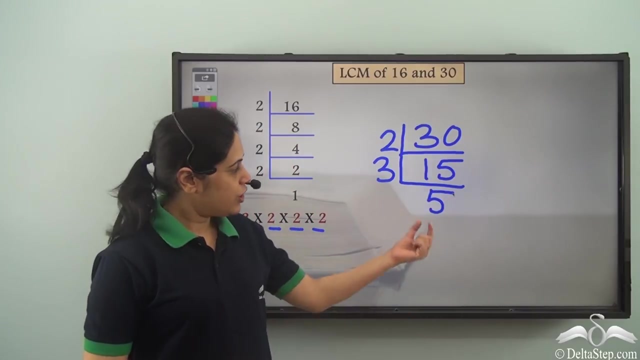 2.. So I get the quotient as 15.. Now is 15 divisible by 2? No, So I move to the next prime number, which is 3.. 15 is divisible by 3, and I get 5.. Now 5.. 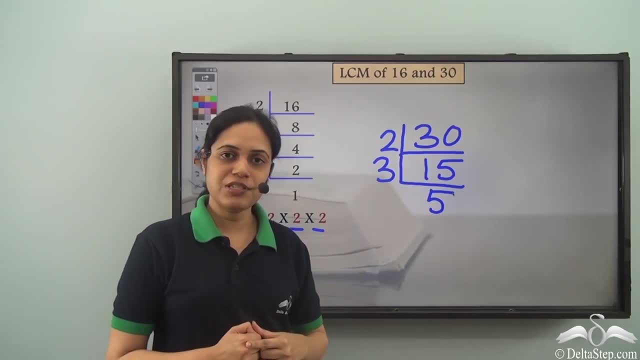 So, since I am dividing by 3, I check with 3 first. Is 5 divisible by 3? No, So I move to the next prime number, which is 5 itself. So I move to the next prime number, which is 5 itself. 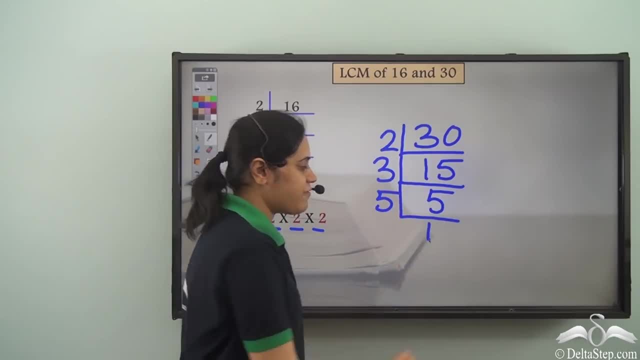 So I check with 3 first. Is 5 divisible by 3? No, So I move to the next prime number, which is 5 itself, And 5 is divisible by 5.. 5 goes into 5 one time, So we have reached 1.. 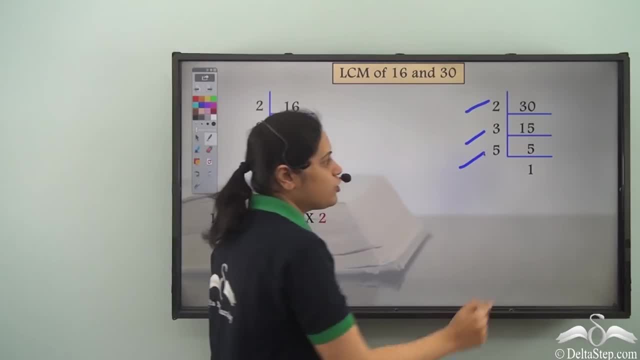 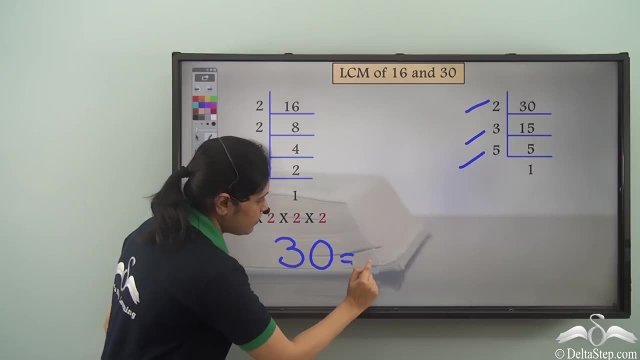 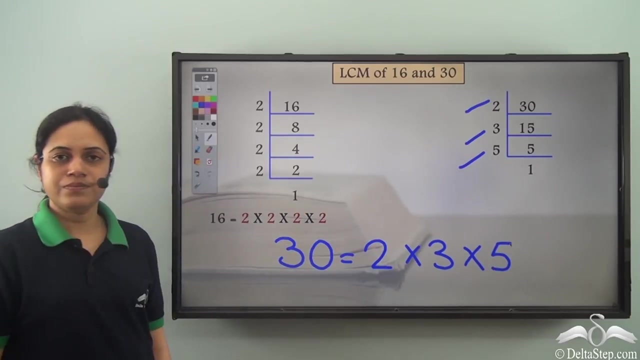 So 30 is 2 into 3 into 5, because these are the divisors. So I can write 30 as 2 into 3 into 5.. So this is what is 30.. Now I have prime factorised 16 and 30.. 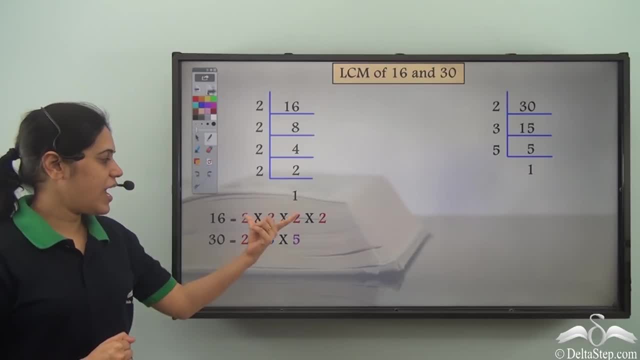 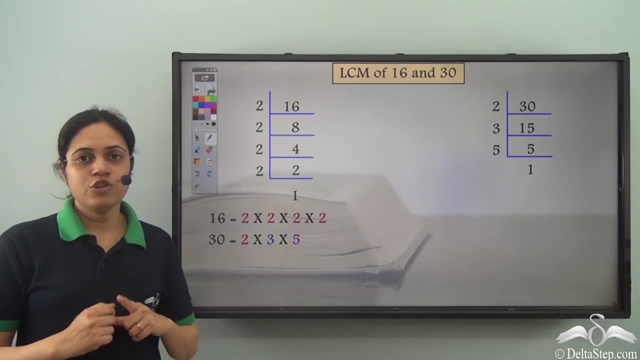 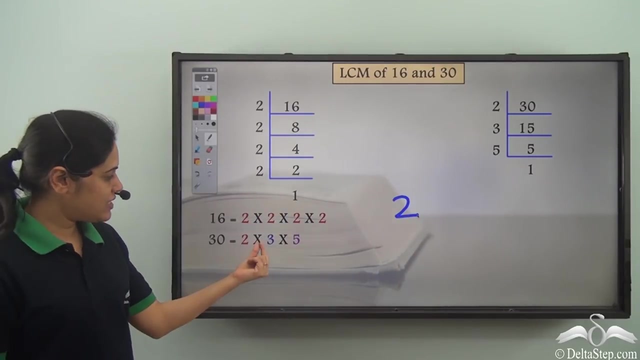 Now, how do I find the LCM? First I need to see what are the different prime factors present in either of them. So I see that there is 2.. So 2 is present. I see that there is a 3 here. 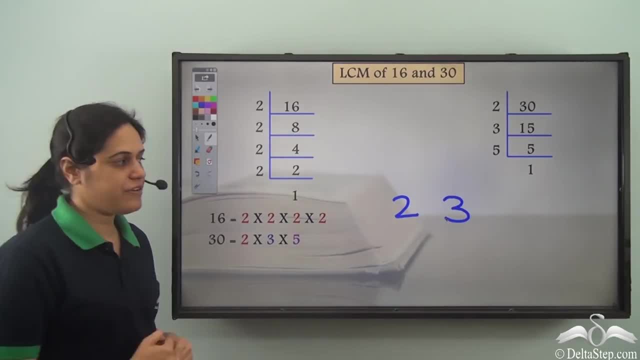 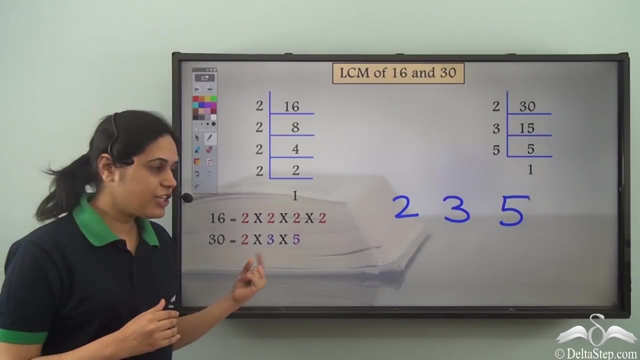 So 3 is present. I see that there is a 5 here, So 5 is present. So I am not taking the prime factors which are present in both. I am taking the prime factors which are present in either of them, Say for example 3.. 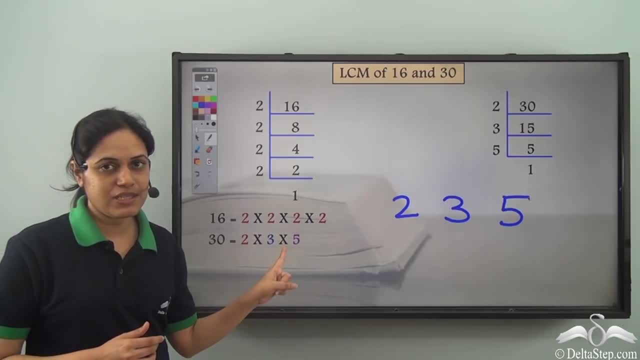 3 is present only in 30 and not present in 16. But still I am writing 3 here 5.. 5 is present only in 30, but not in 16.. Still I am writing 5 here, 2.. 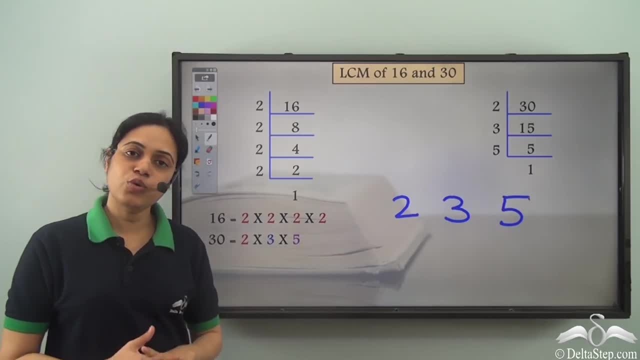 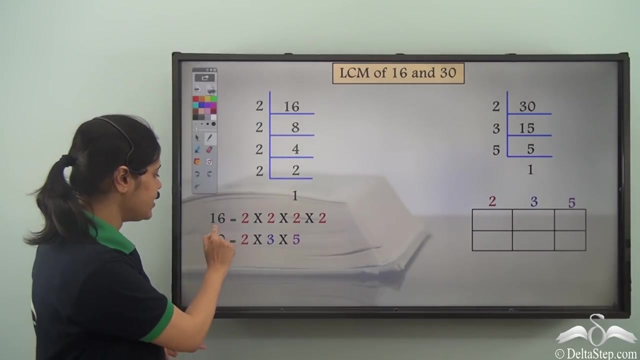 2 is present in both. I am writing 2 as well, So I am taking the prime factors which are there in either one or both. So I make a table like this. Now, how do I fill this table? So over here I write: how many times is 2 present in 16.. 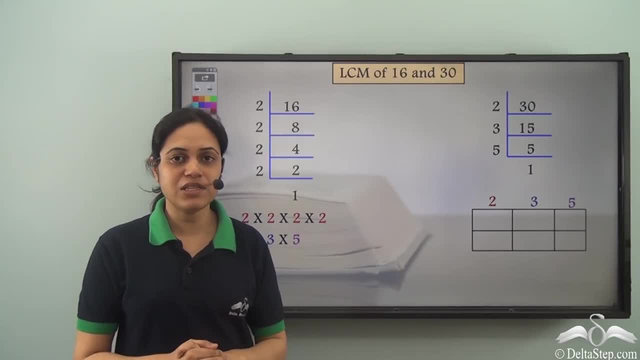 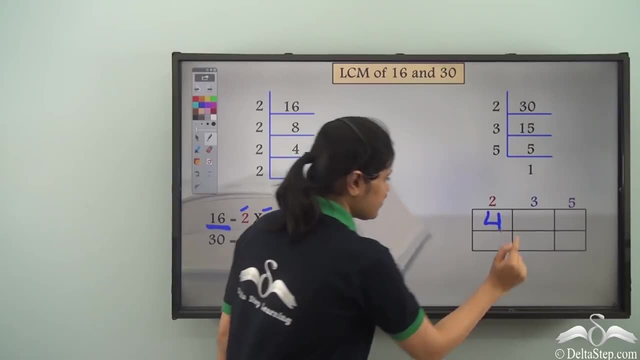 So this prime factor: 2.. How many times is 2 present in 16?? How many times is it present in 16? 1,2,3,4.. 4 times. How many times is 3 present in 16?? 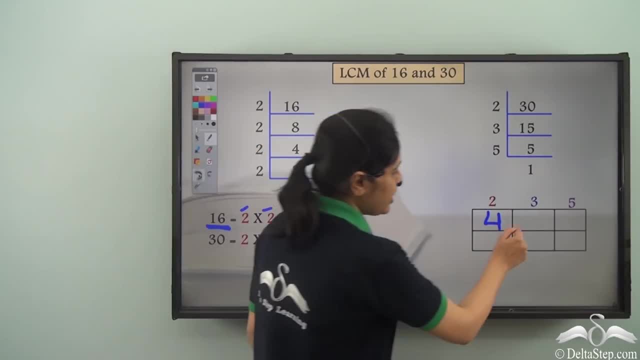 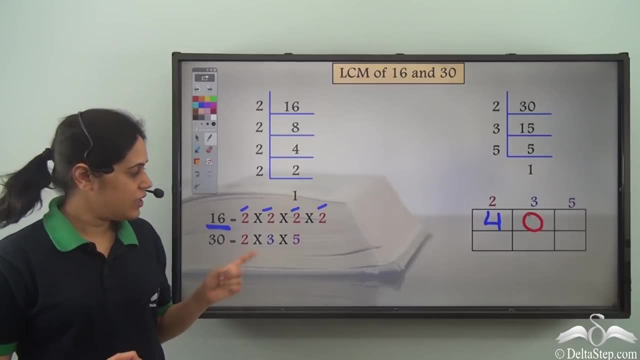 3 is not present in 16.. So 3 is present 0 times. How many times is 5 there in 16?? There is no 5 in the prime factorization of 16.. so five is present zero times. so this is what i have now. if i look at 30, how many times is? 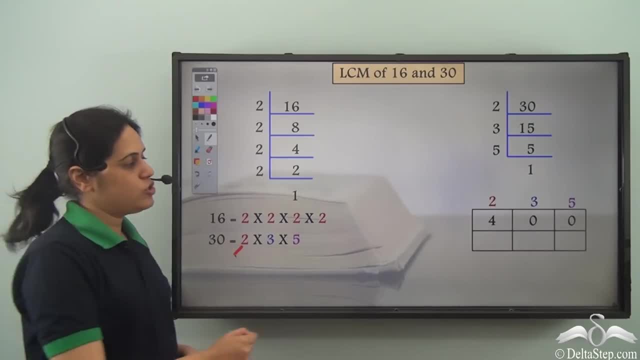 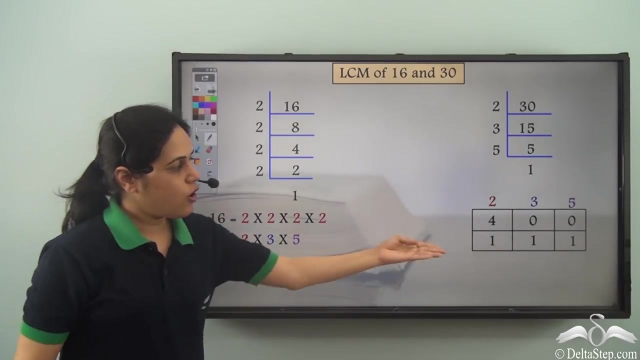 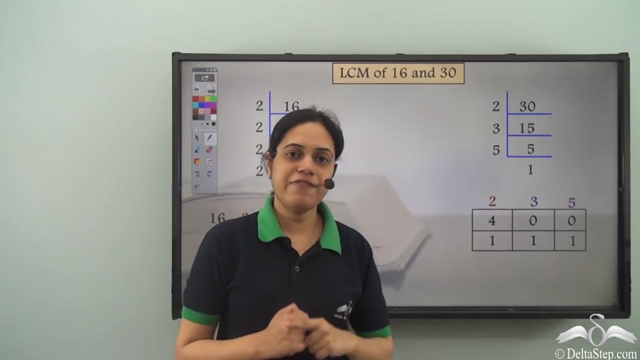 2 present in 30 one time, so 2 is present once. how many times is 3 present in 30? just once. so i write 1 here. how many times is 5 present in 30? one time? so 1. so in 30 all three are present once. now what do i do with this? i consider all the prime factors. 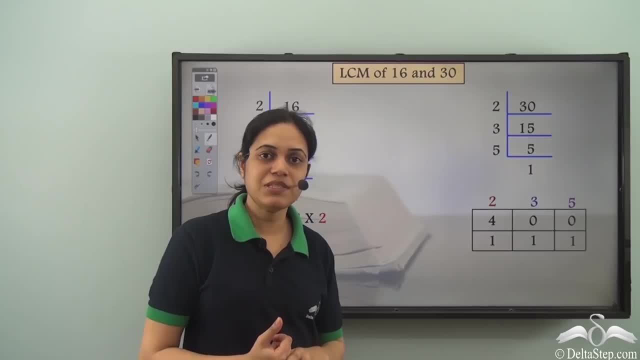 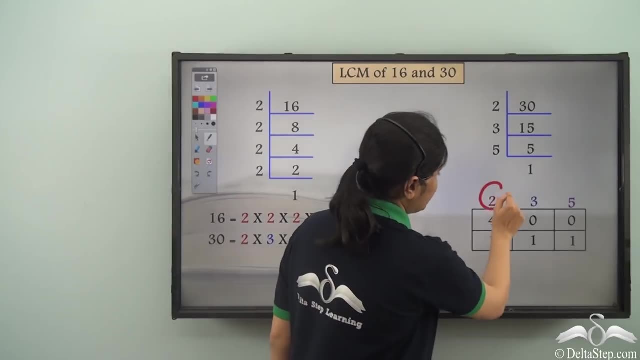 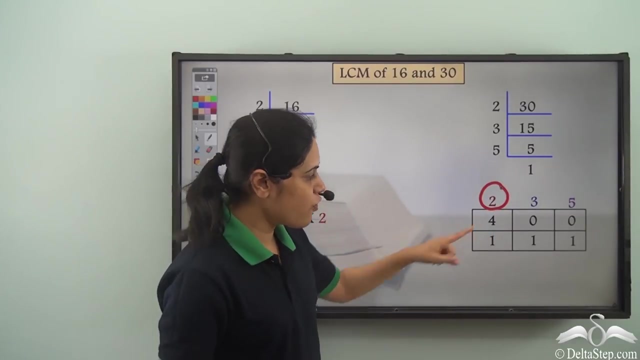 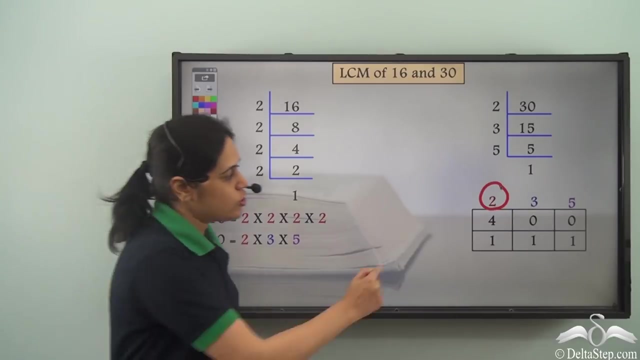 and take the maximum number of times they are present in either of them. what do i mean by that? so first i take 2 and i see the maximum number of times it is present. that is 4. 2 is present four times in 16 and just one time in 30, so i consider 4. so this 4 is considered. 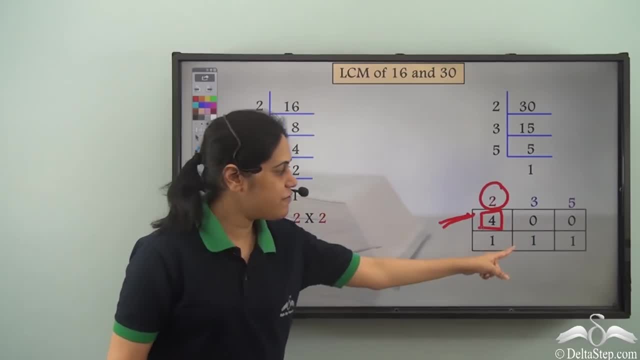 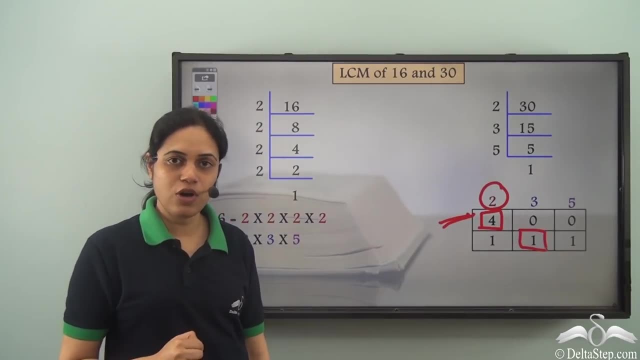 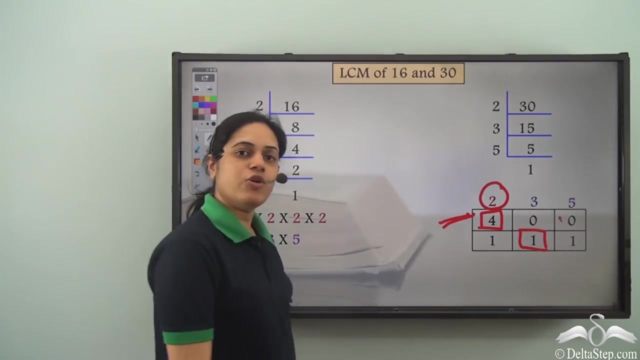 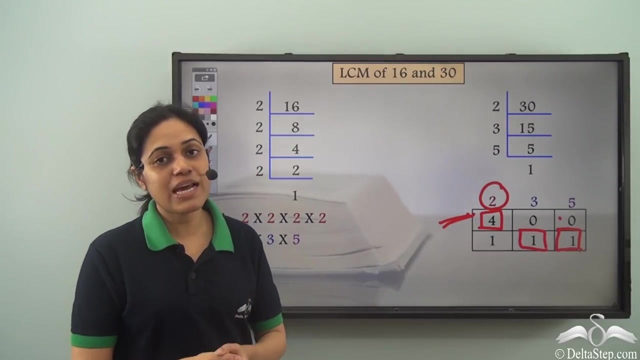 3 is present 0 time in 16 and 1 time in 30, so i consider 1 because 1 is greater than 0. i need to consider maximum time for 5. it is present 0 time in 16 but 1 time in 30, so i consider 1 because i am considering. 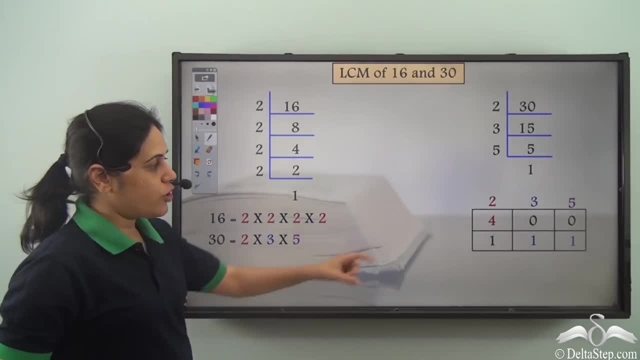 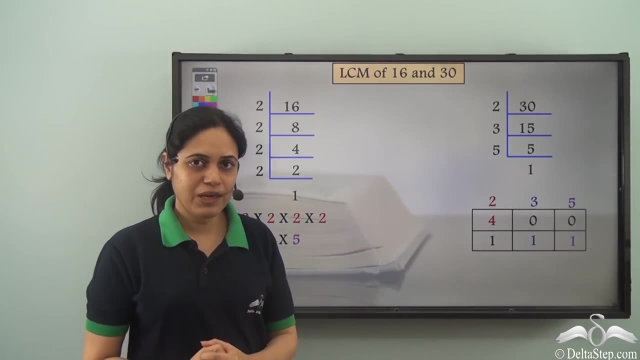 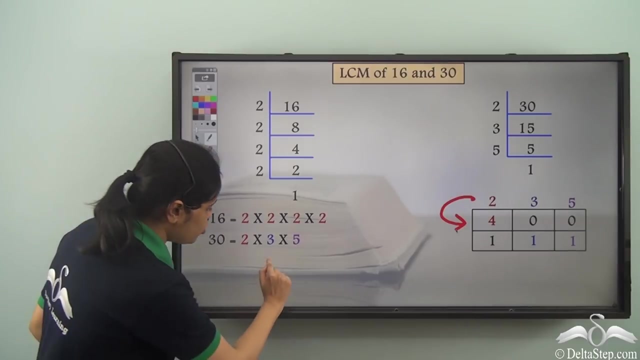 maximum number of times. so for 2, so i have 4. for 3 i have 1, and for 5 i have 1.. what do i mean by this? i consider 2, 4 times so 2, and for 5 i have 1. what do i mean by this? i consider 2, 4 times, so to. 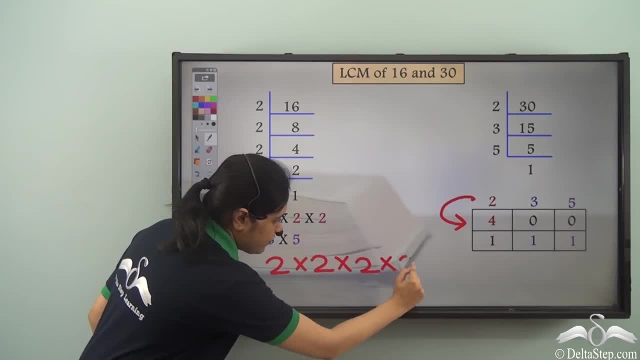 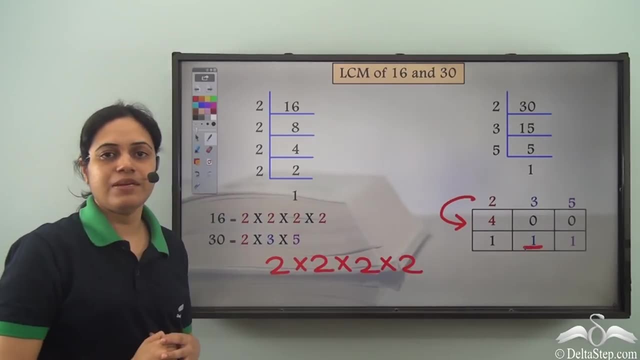 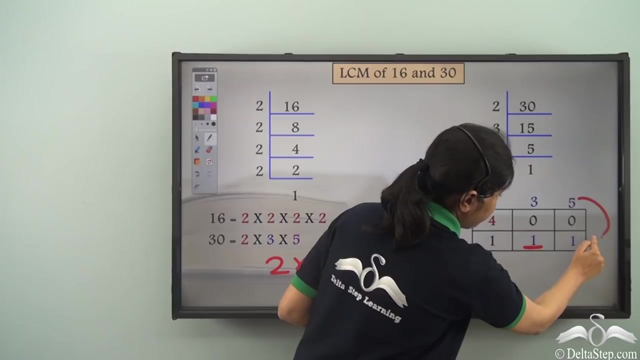 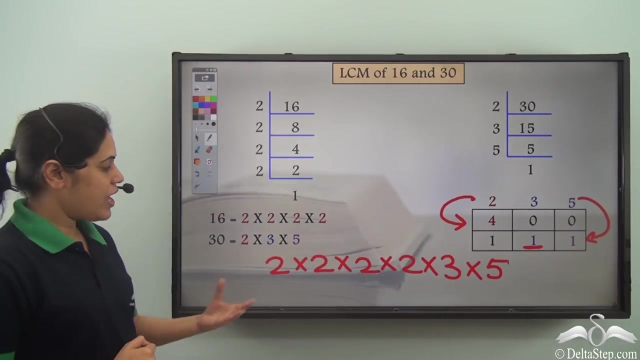 4 times. 2 multiplied with itself 4 times, I consider 3 one time. So now I multiply 3 one time and I consider 5 one time. So I multiply 5 one time and this is what is my LCM. So 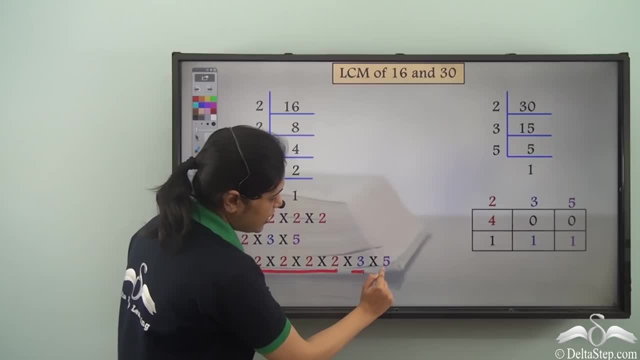 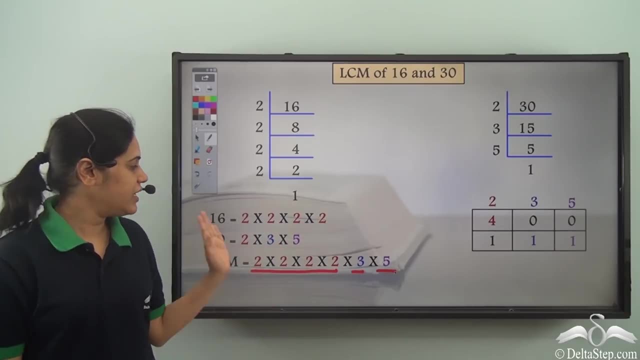 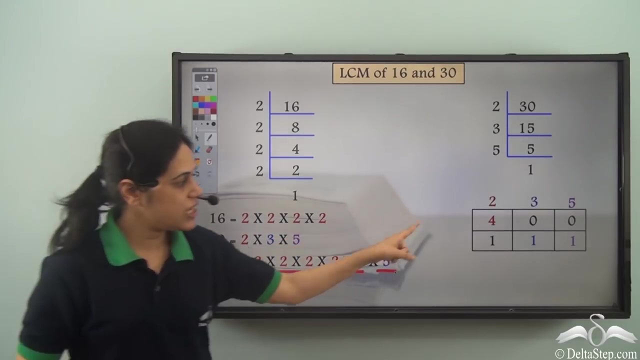 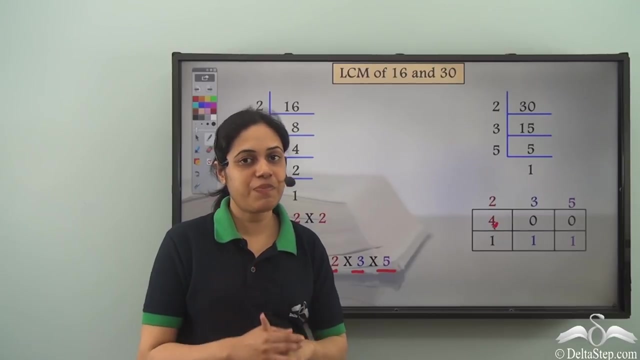 2 four times, 3 one time and 5 one time. I take up the different prime factors which are present in either of the numbers, I find the maximum number of times they are present. So see, I am not adding 4 and 1.. I am considering the maximum number of times it is present. 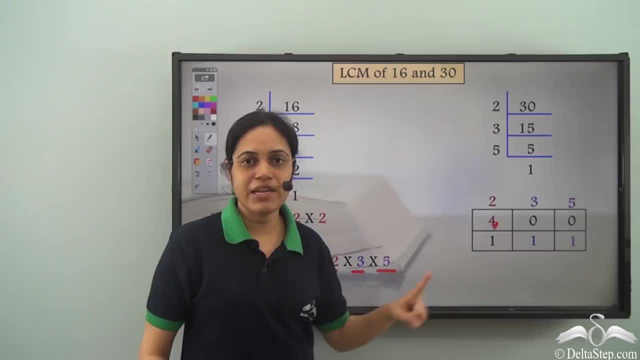 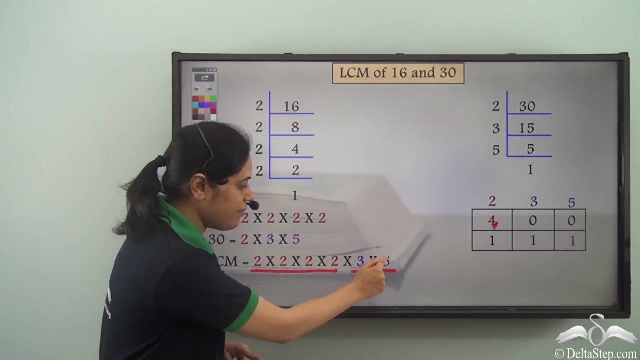 in any one. I don't add 4 and 1 and take 5.. Nor do I subtract. I see which is the higher number between 4 and 1.. 4. So I consider 2 four times, So 2 four times, 3 one time and 5 one time. And if you multiply this, you 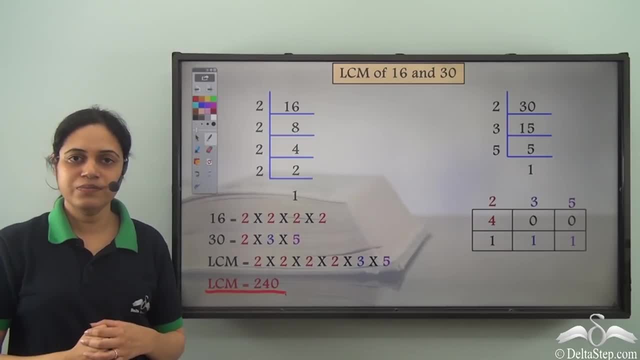 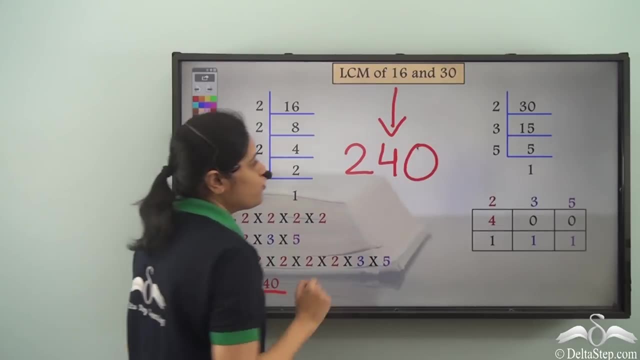 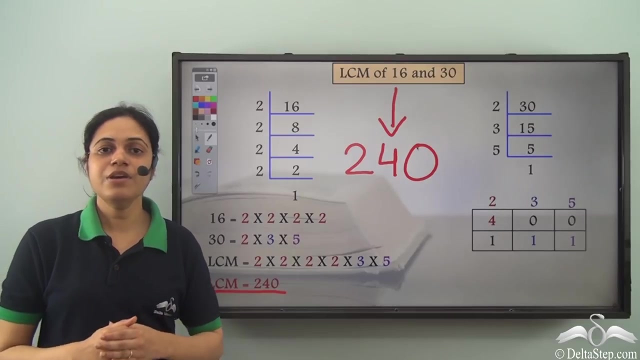 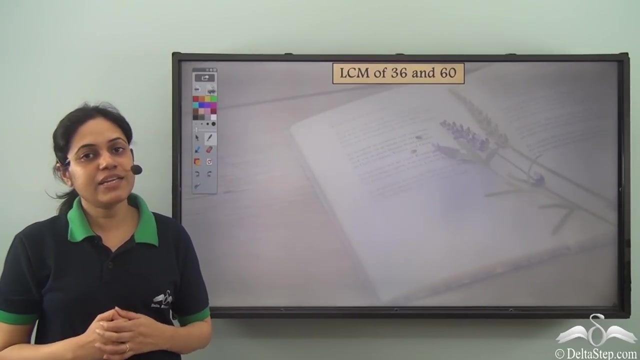 will get the LCM as 240.. So the LCM of 16 and 30 is 240.. That is 240, and this is how we can find the LCM using the prime factorization method. So now can you find the LCM of 36 and 60 using the prime factorization method. So what is? 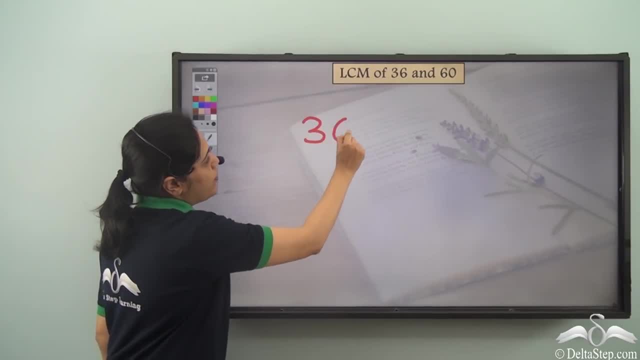 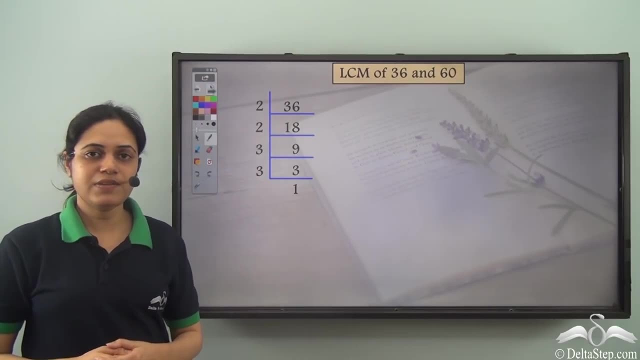 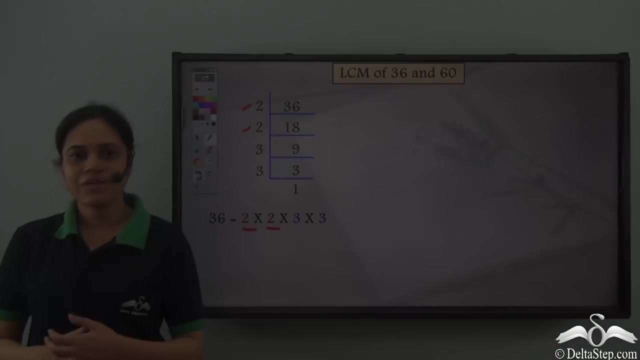 the first step. First I need to prime factorize 36.. So if you prime factorize 36, this is what you get, So you can write 36, as I have two 2s, so 2 into 2, and I have two 3s, so I have two. 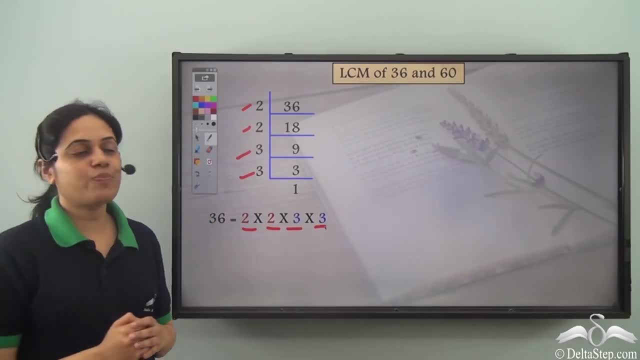 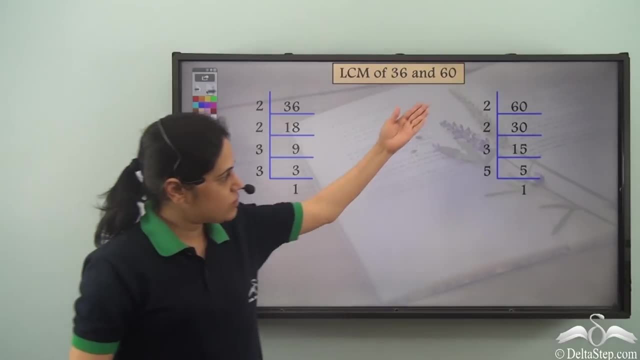 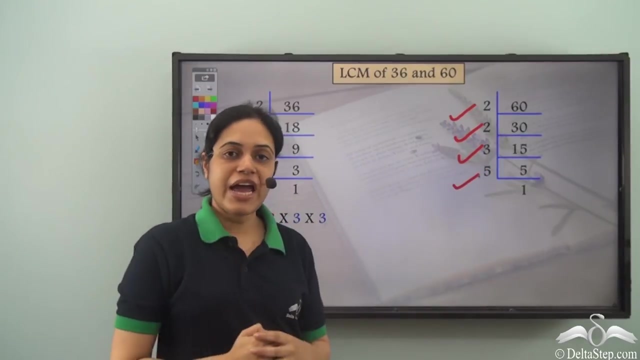 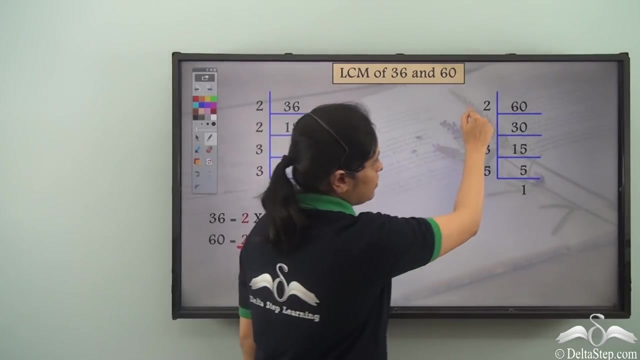 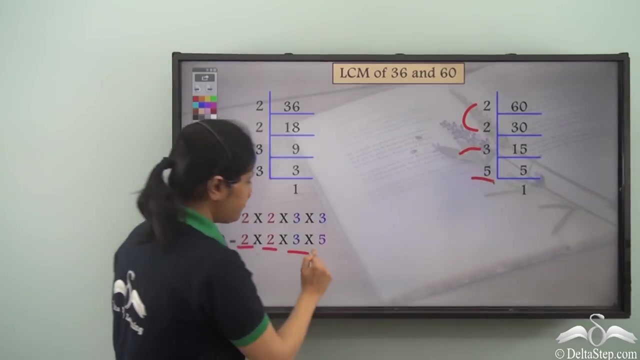 3s here. Next, I need to prime factorize 60, so this is what you get when you prime factorize 60. These are the divisors, so you can write 60 as a product of these numbers. So 60 is 2 into 2,, 2 into 2, into 3, into 3, into 5, into 5.. 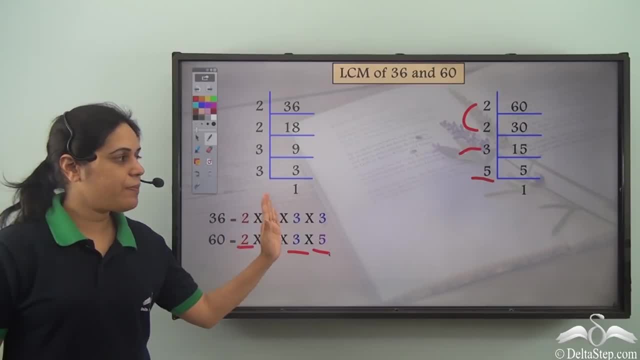 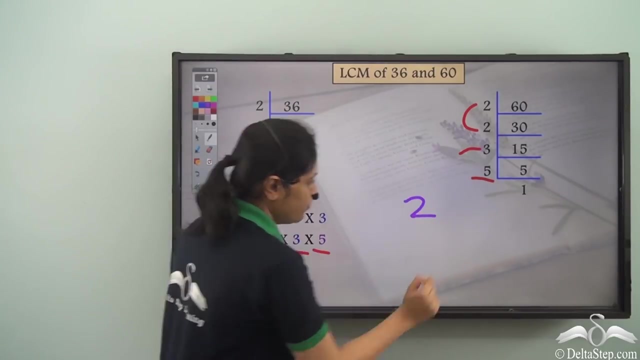 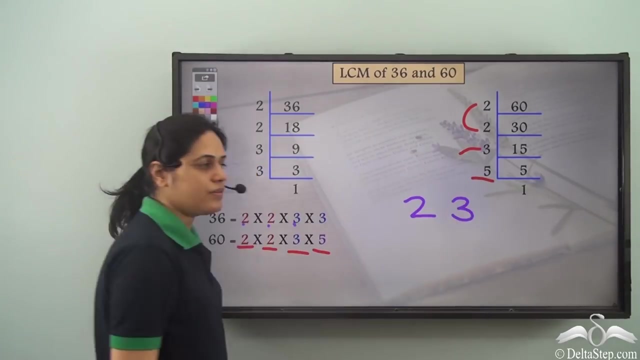 Now, what is the next step? I consider the prime factors which are present in either of them. So what are the prime factors which are present in either of them? So first I see that there is a 2 here, So I write 2, there is a 2,, I have already taken 2, there is a 3, so I write 3, there. 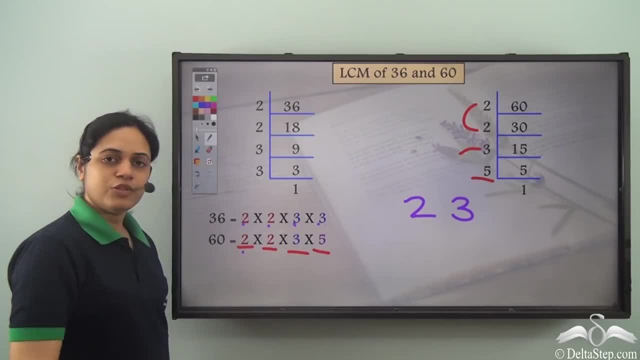 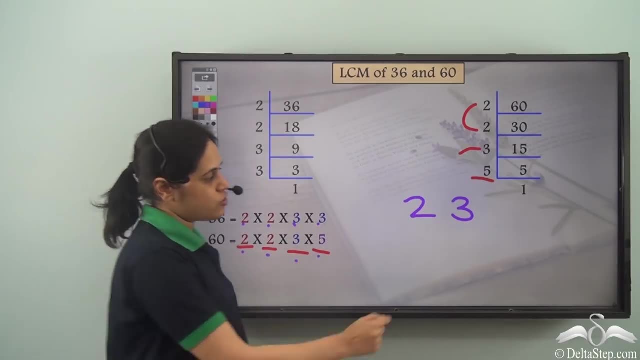 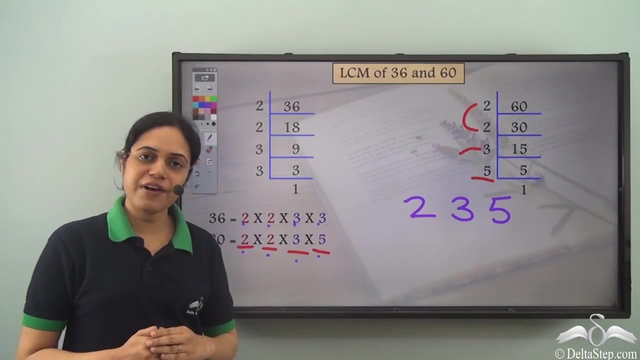 is a 3, I have already taken 3, 2, 2 is taken, 2, 2 is taken 3,, 3 is taken, 5, so I take 5.. So the different prime factors I have are 2,, 3 and 5.. 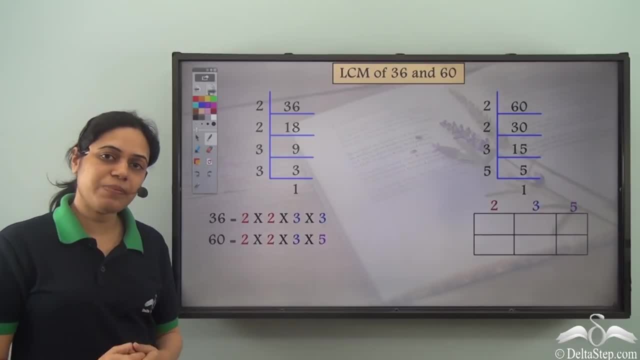 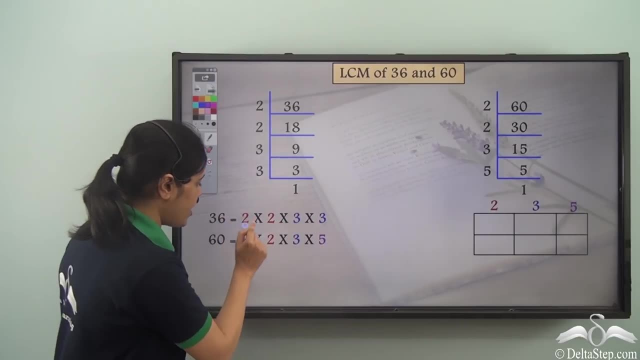 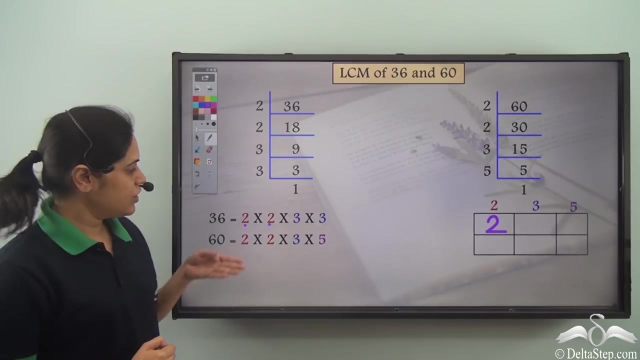 Now I need to find how many times are they present. So 2, how many times is it present in 36?? 1,, 2, it is present 2 times. What about 3?? How many times is 3 present in 36?? 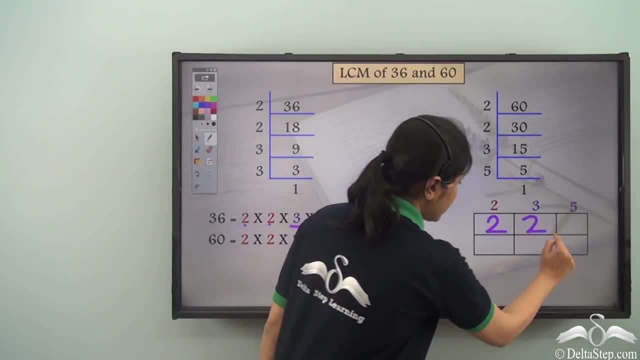 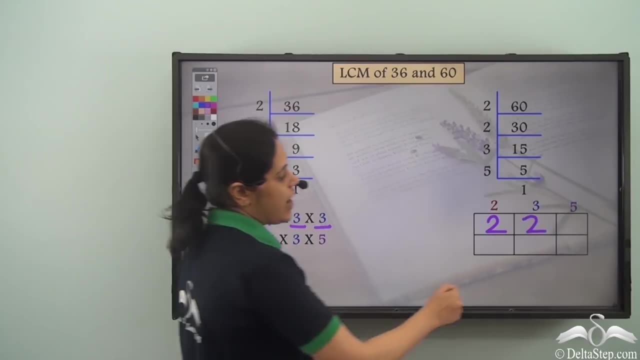 1, 2.. So 3 is present, So 3 is present. So 3 is present 2 times. And what about 5?? 5 is not present in 36 at all. So 5 is present 0 times. 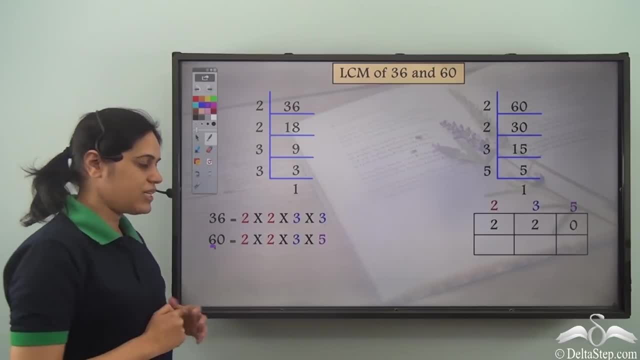 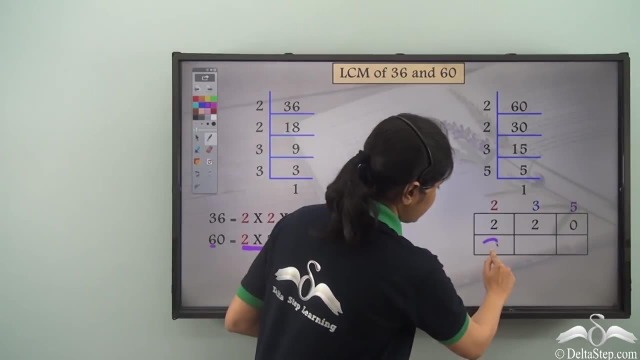 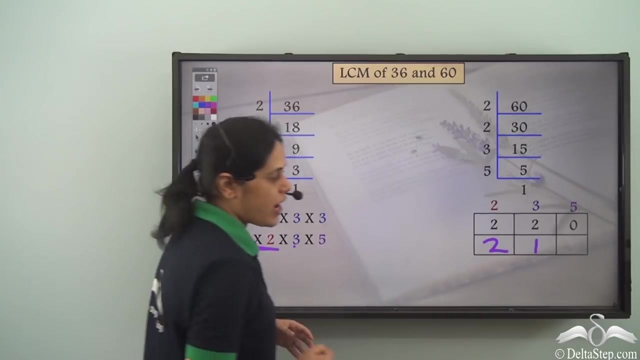 So this is what I have Now. let us consider 60. How many times is 2 present in 60?? 2 times, So I write a 2 here. How many times is 3 present? 1 time, So I write 1.. 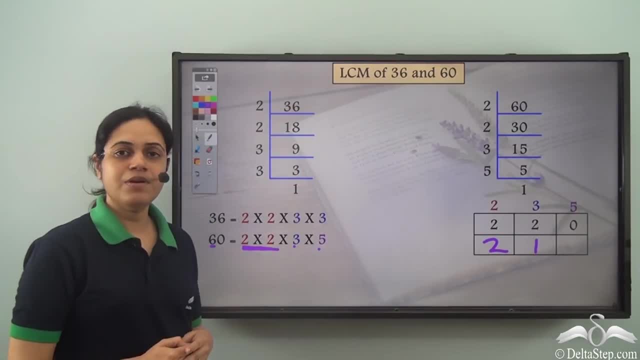 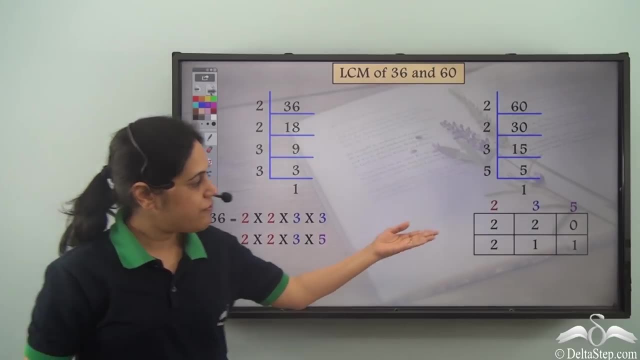 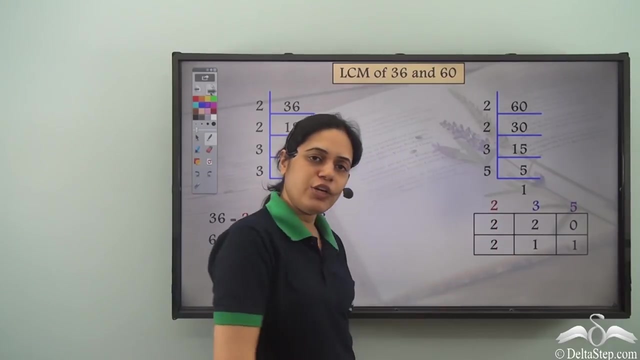 How many times is 5 present? 1 time, So I write a 1 here. What is the next step? Well, find the maximum corresponding to each prime factor. So for 2, I have 2 and 2.. So the maximum can be this or this. 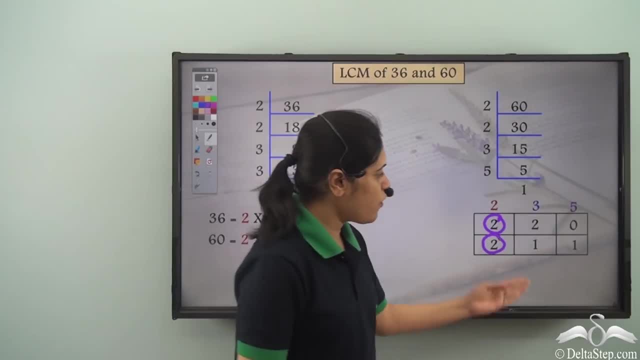 It doesn't matter, because 2 is equal to 2.. For 3, the maximum is 2.. Because between 1 and 2, the maximum is 2.. So I write 1 here. So 1 and 2, 2 is greater. 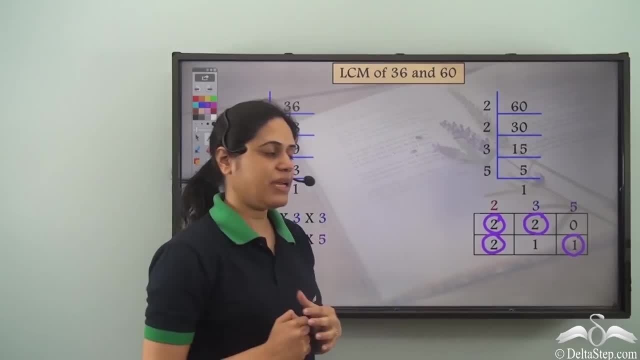 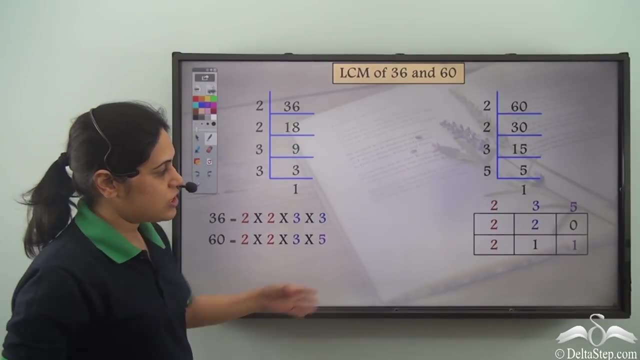 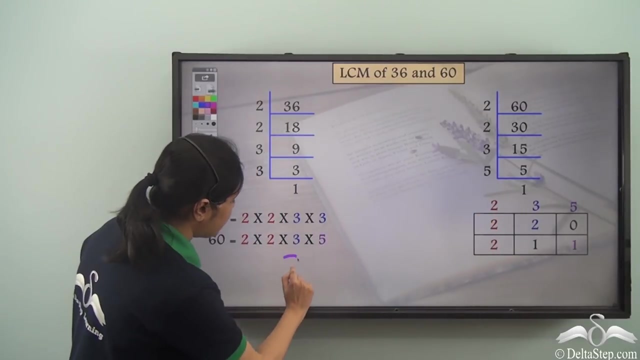 For 5,, the maximum number of times is 1, because between 0 and 1,, 1 is greater. So this is what I have. So I need to consider 2, 2 times. So I multiply 2, 2 times. 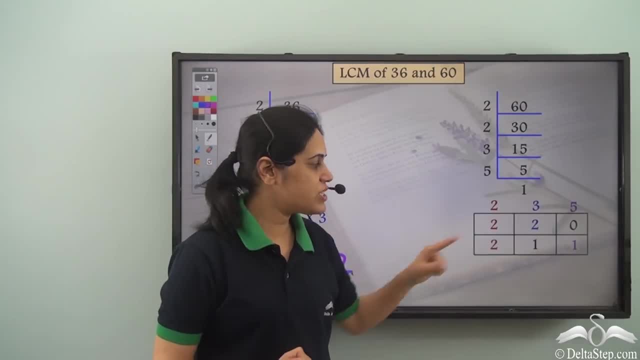 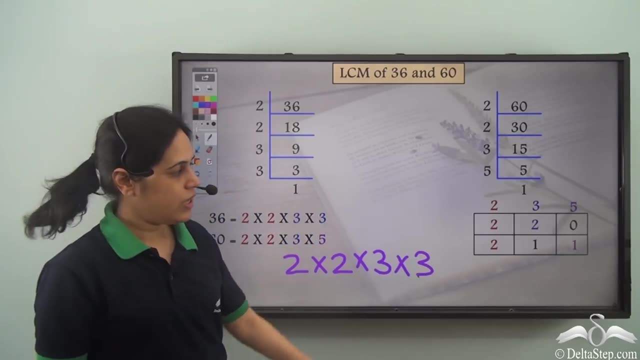 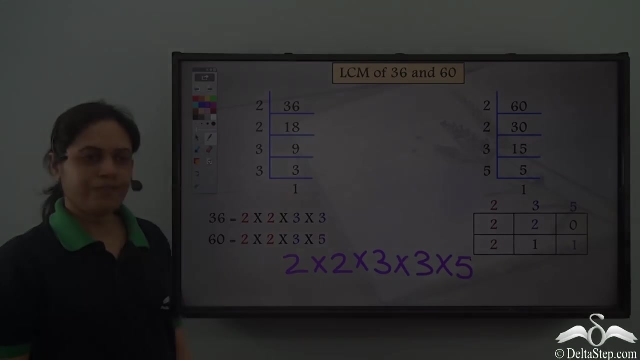 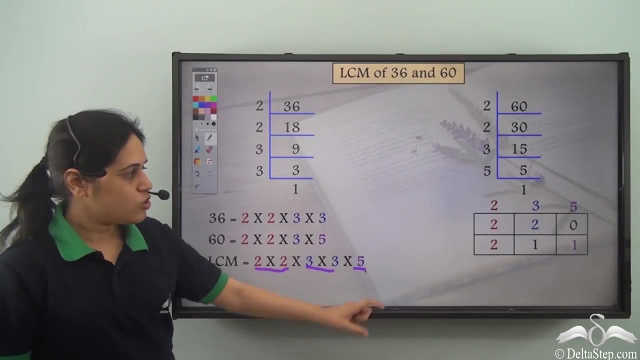 3, 2 times, because 2 is greater. So I multiply 3 also two times. So 1, 2 and I consider 5 one time. So I multiply 5 one time. So I have 2 two times, 3 two times and 5 one time. So note, I am not adding them, I am. 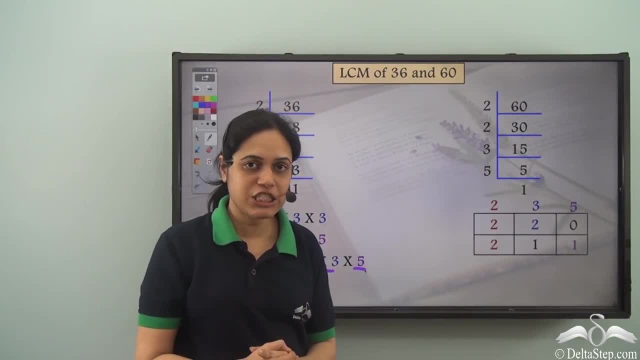 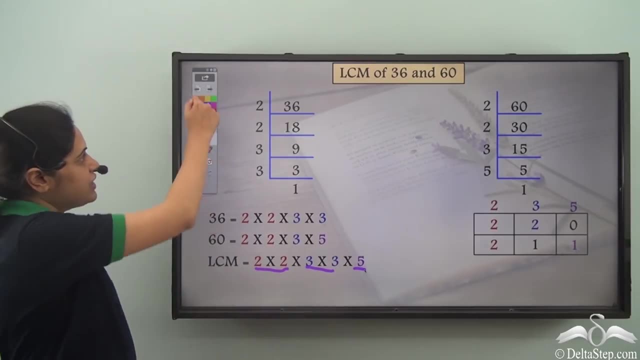 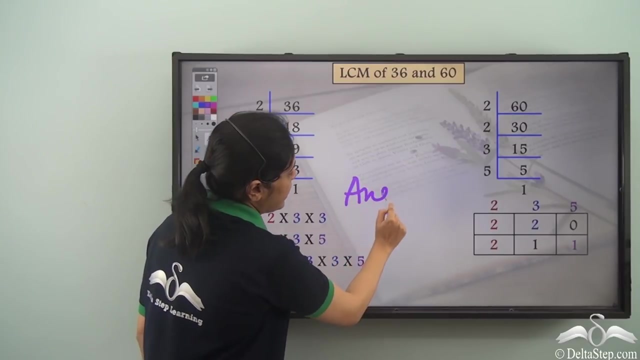 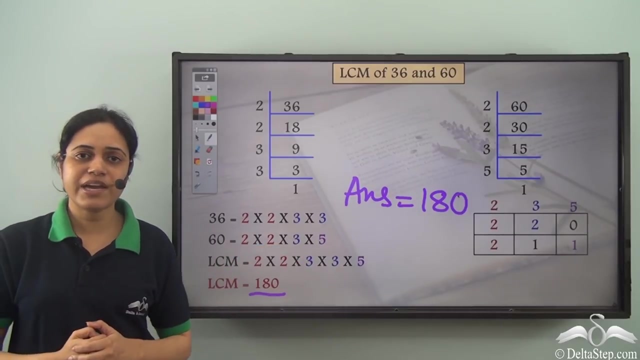 finding the maximum corresponding to each prime factor and multiplying it that many number of times. And if you multiply these you get the LCM as 180.. So the answer or the LCM is 180. So see how easily you can find it using prime factorization method. Also observe: 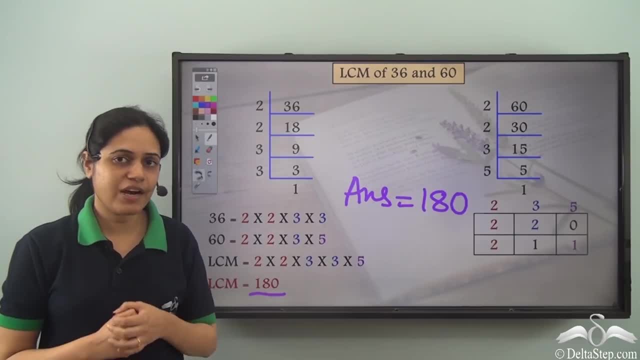 something. What is LCM? LCM is 180.. Is 180 equal to 36 into 60?? No, LCM is not equal to the product of the numbers, So it is a very common mistake to think that LCM is actually the product or the. 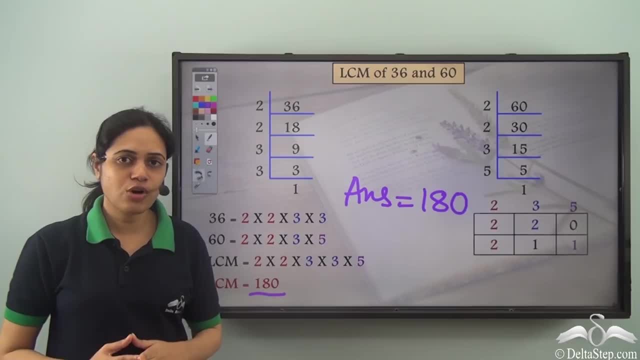 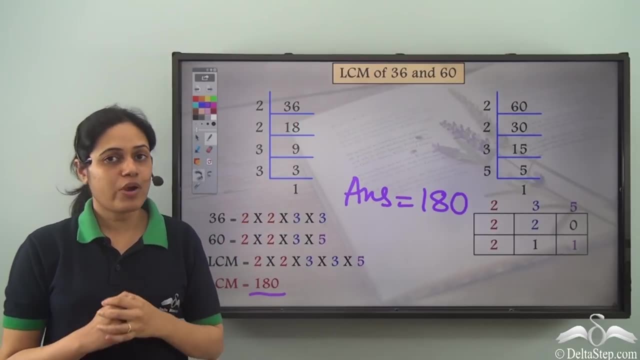 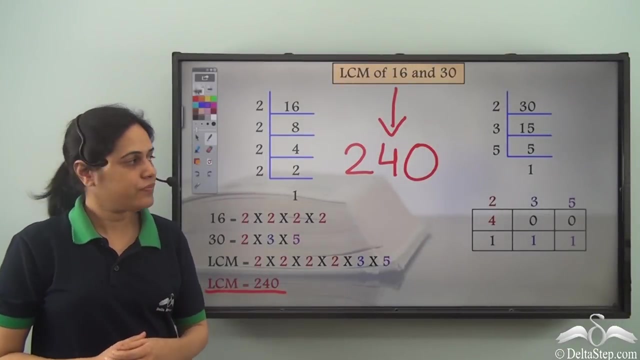 multiplication of the numbers. But it is not so. So we can easily see that 180 is not equal to 36 into 60. So LCM is not equal to the product of the numbers. Also, observe something: Is 240 equal to 16 into 30?? 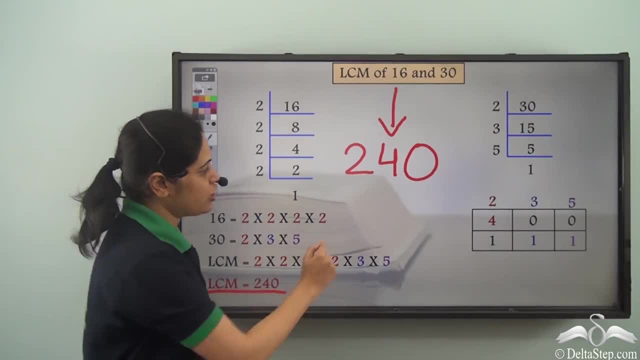 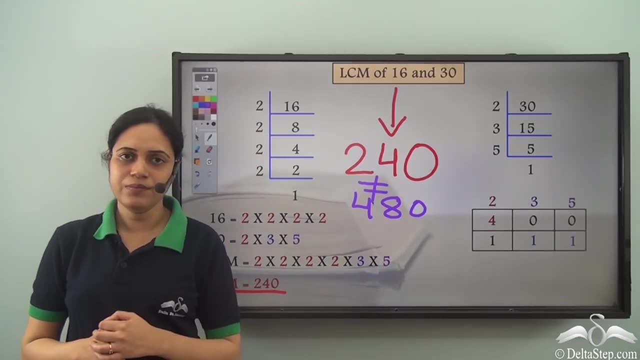 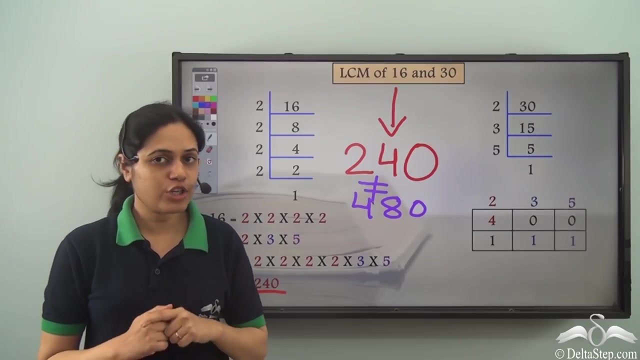 No 16 into 30 is actually 480, which is not equal to 240. But the LCM is 240.. So the LCM is not equal to the product of the numbers. It is a very common mistake to think that. 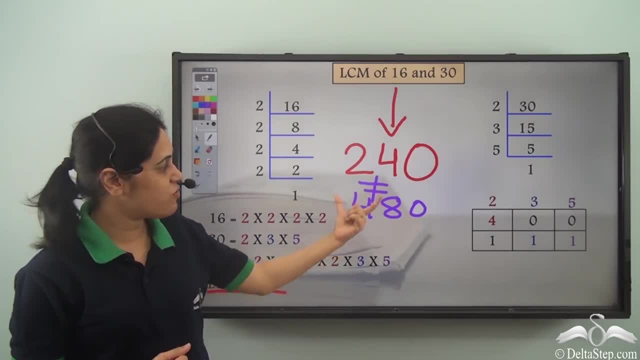 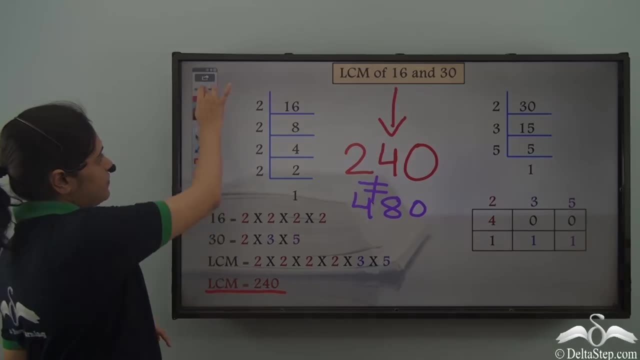 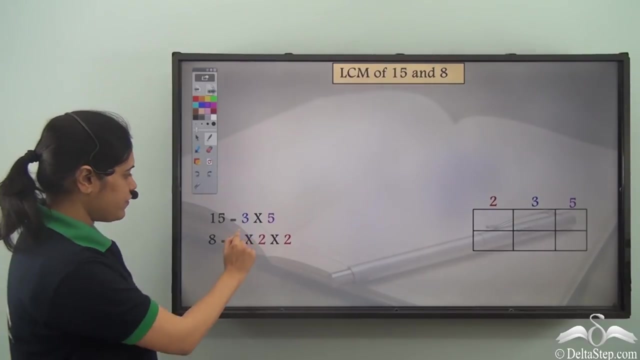 LCM is actually the product of the numbers. But, as we can clearly see, LCM is not equal to the product of the numbers. But consider this case. So suppose we need to find the LCM of 15 and 8.. So 15 can be prime factorized in this manner. 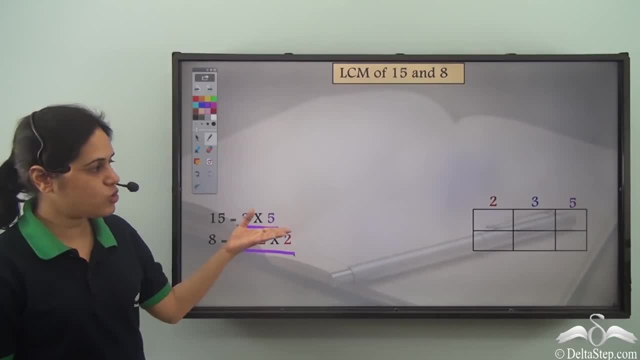 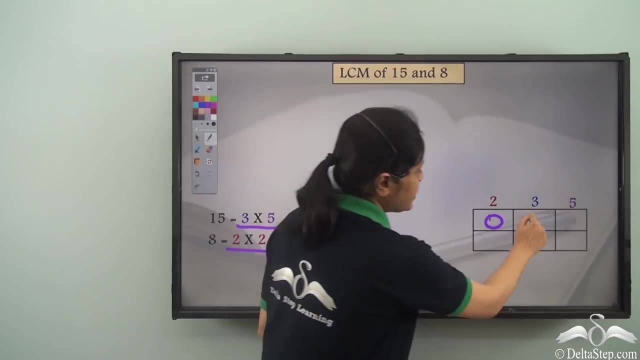 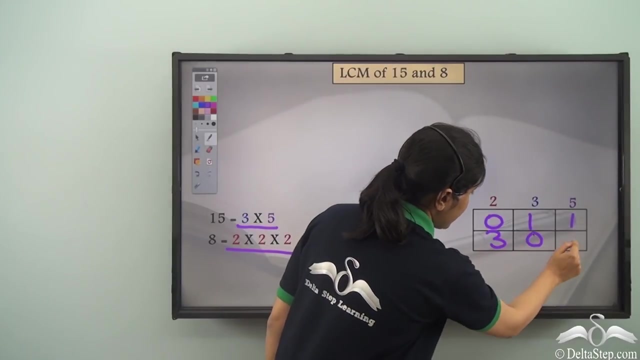 and 8 can be prime factorized in this manner as 2 into 2 into 2.. Now, 2 is not present in 15.. 3 is present one time and 5 is present one time For 8,. 2 is present three times, 3 is not there. 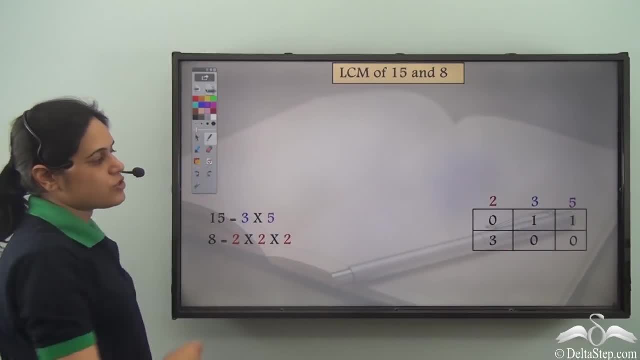 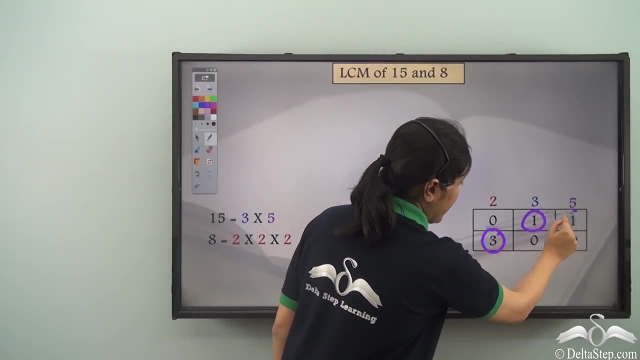 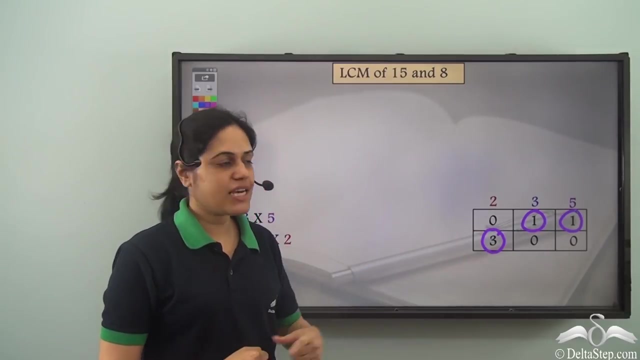 and 5 is not there. So this is what I have To find, the LCM. I consider 3 from here, 1 from here and 1 from here. So what does it mean? 2 multiplied three times, 3 multiplied one time? 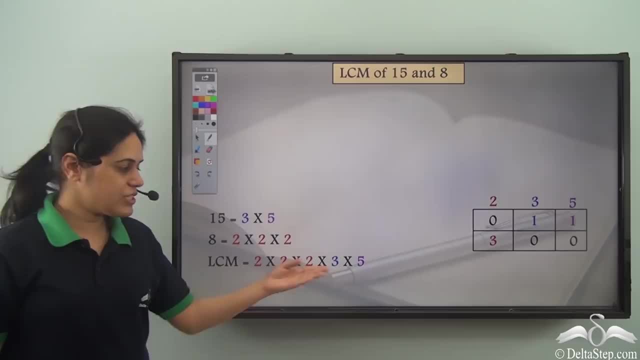 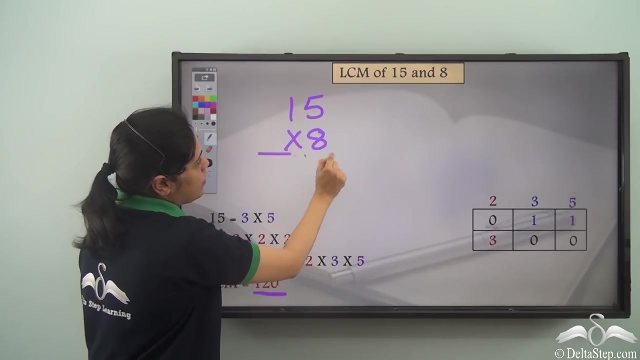 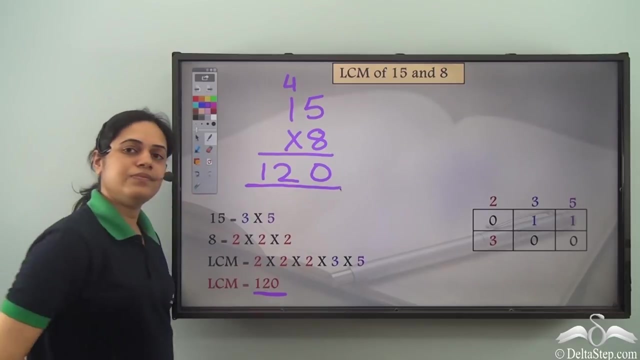 and 5 multiplied one time. This is what I have Now. if you multiply these, you will get 120 as the LCM. What is 15 into 8?? So 15 into 8 is also 120. So in this case, LCM is actually equal to the product of. 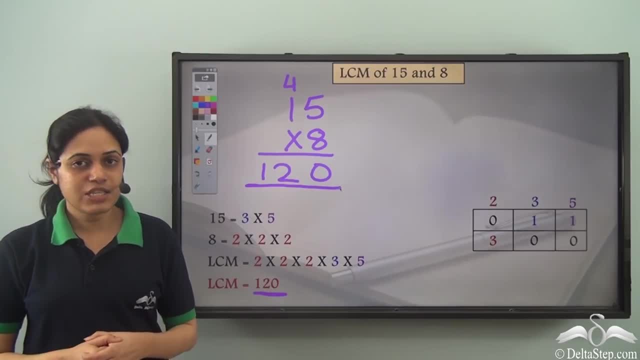 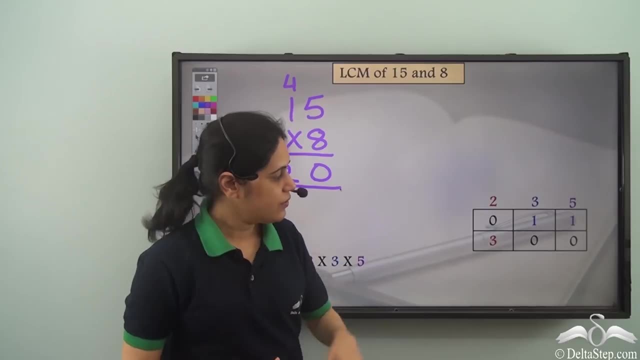 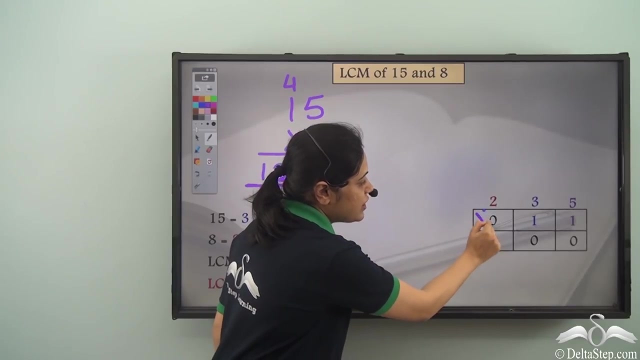 two numbers. Why is it? It is because 15 and 8 have no common prime factor. See, they have no common prime factor. 2 is present in 8, but it is not present in 15.. 3 is present in 15, but not present in 8.. 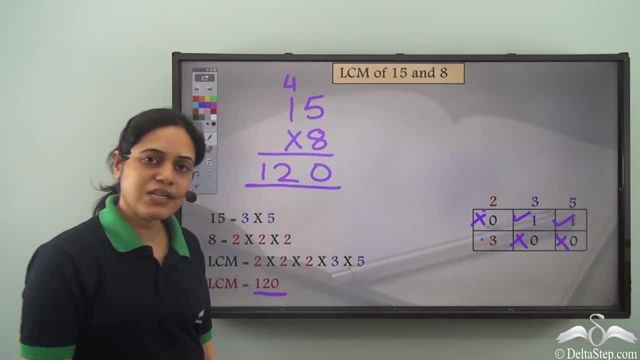 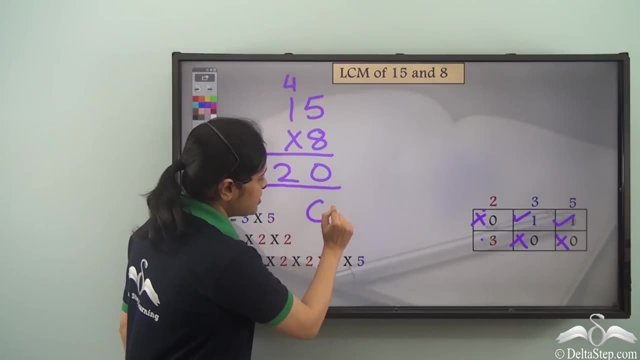 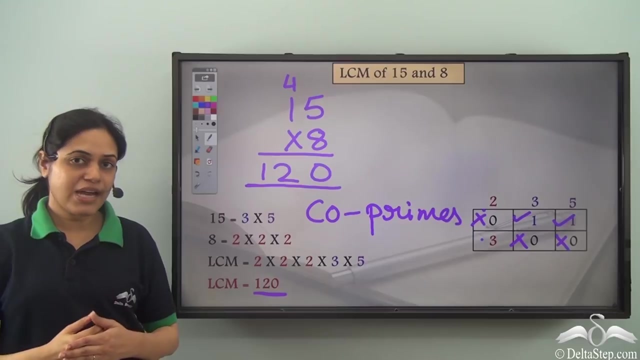 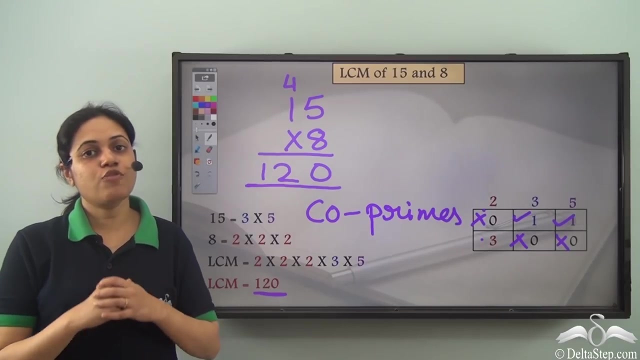 5 is present in 15, but not present in 8. So what do I call such numbers? Do you remember? Such numbers are called co-primes because they don't have any common factor other than 1.. So co-prime cut. So for co-prime numbers, LCM. 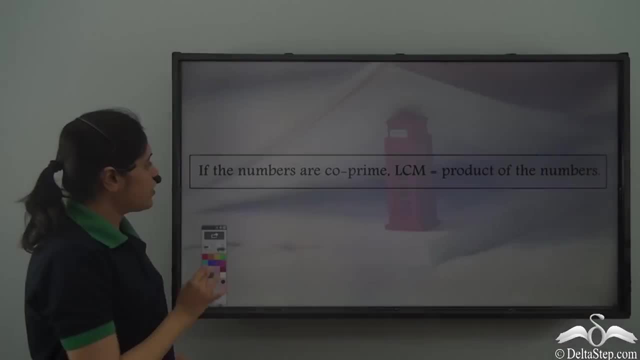 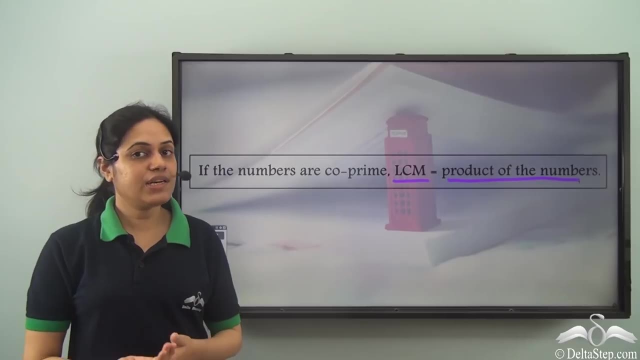 is equal to the product of the numbers. So if the numbers are co-prime, then LCM is equal to the product of the numbers. But in no other case will the LCM be equal to the product of the numbers, Only when the numbers are co-prime. 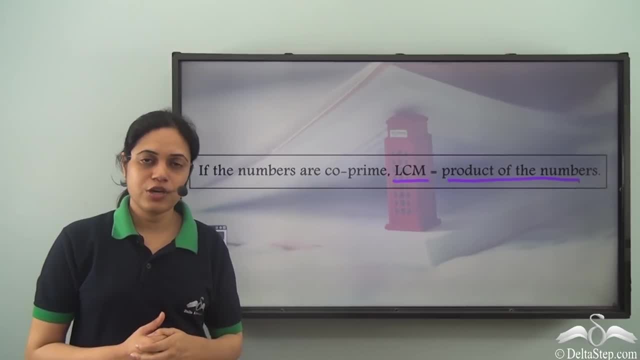 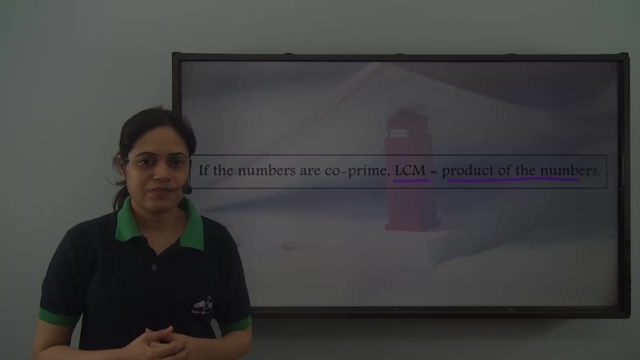 then LCM is equal to the product. So this is how you can find the LCM using the prime factorization method. So take up different numbers, find their LCM using this method till you get them all correct. If you like this video, then subscribe to our channel. 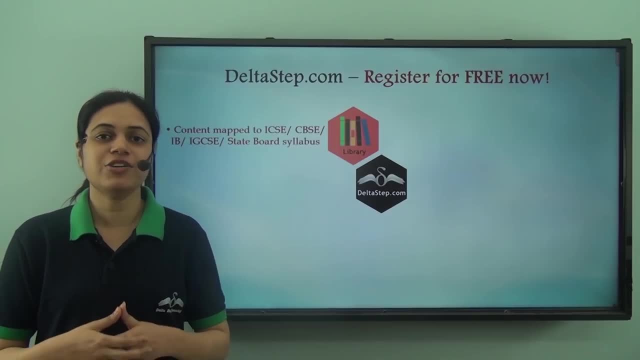 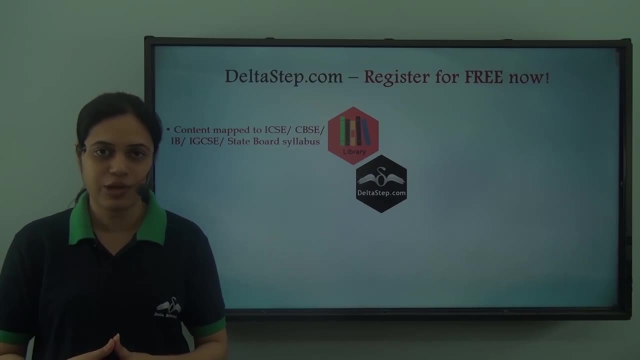 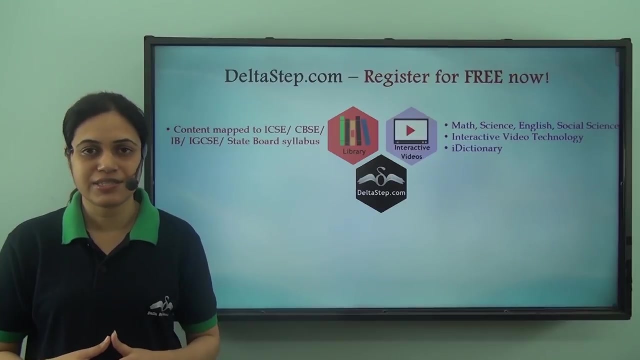 And also register for free at deltastepcom to get all the learning resources as per CBSE, ICSE, IB, Cambridge or any other curriculum. Over 5000 amazing lectures on Maths, Science, English and Social Science. Our unique interactive video technology keeps you engaged and our iDictionary feature. 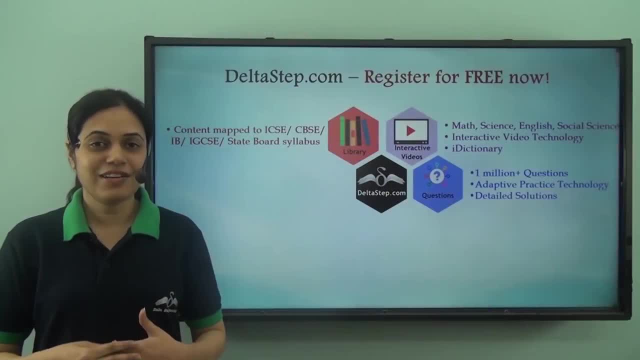 allows you to quickly revise any concept. Master each topic at your own pace with our adaptive practice technology and 1 million plus questions. Get instant answers and detailed solutions. Be exam ready by taking unlimited mock tests, performance analysis along with actionable feedback. Personal tutors to resolve the slightest. 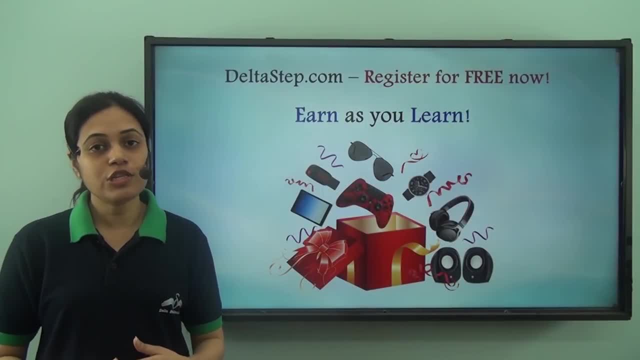 of your doubts. And that's not all. You can also win exciting prizes like PlayStations, iPads, watches and many more, along with certificates through our Earn as you Learn program. So at deltastepcom, learning is not just fun and easy, it is rewarding too. So register for free now.